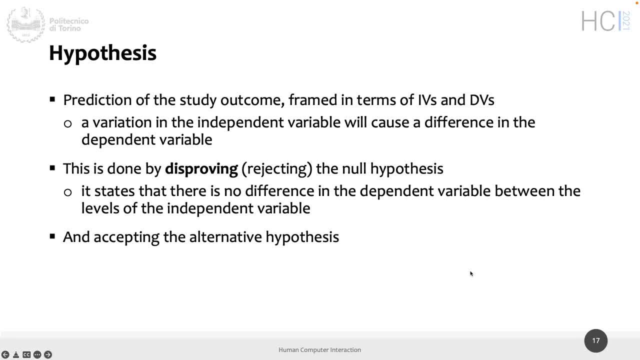 about variables last time and the overall plan and execution Of control experiment. That we said is more hypothesis based, more scientific, And we defined that there are two main kind of variables: The independent variables, That is, the things we manipulate to demonstrate our point, And the dependent variables That are typically. 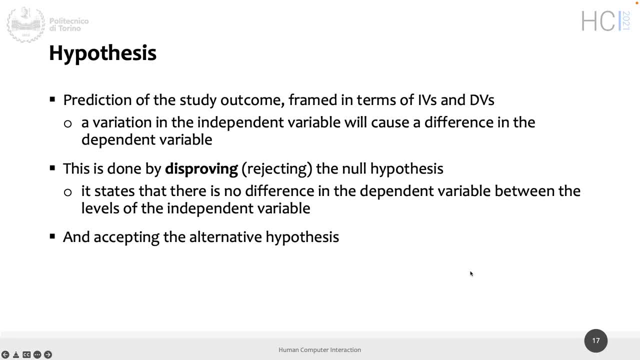 the things that we measure according to the changes to the independent variable, And we also said there are other three types of variables- Confounding variable, Control variable And random variable- That we cannot manipulate. consider according to the different cases And we 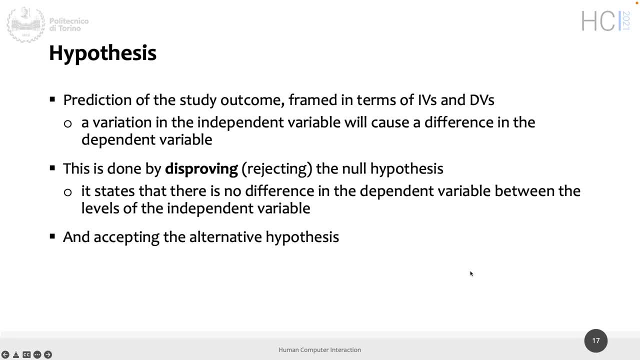 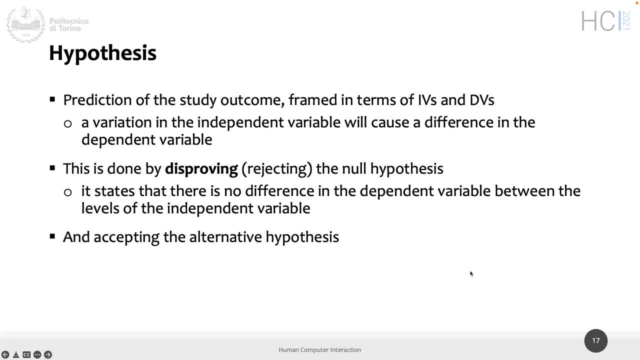 Which is the outcome, what we want to demonstrate- And until this point we said that we want to demonstrate that version 1 of an interface is better in some measurable way than version 2. And we defined that as our hypothesis, our goal. 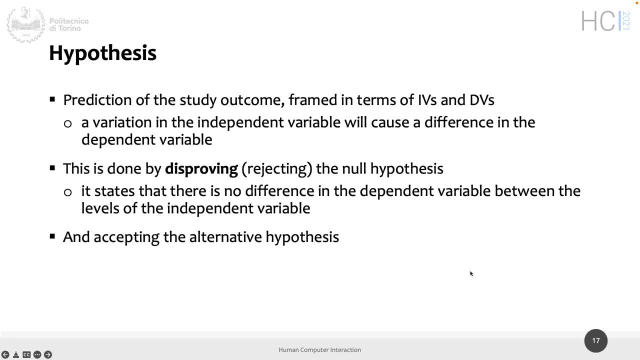 And here now we are going to define better this hypothesis, moving from the handcrafted goal that we defined up to now to a more structured way of defining an hypothesis. So what is the hypothesis? The hypothesis is the prediction, our prediction of the study outcome, framed in terms of independent 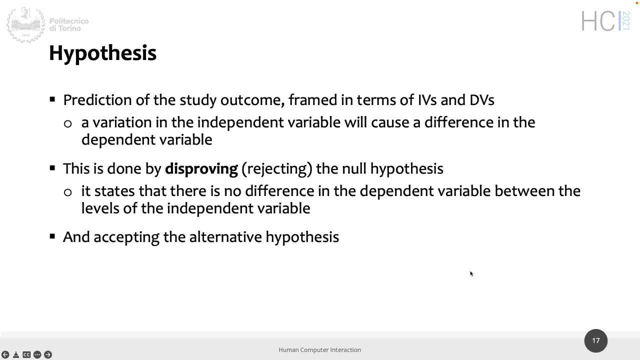 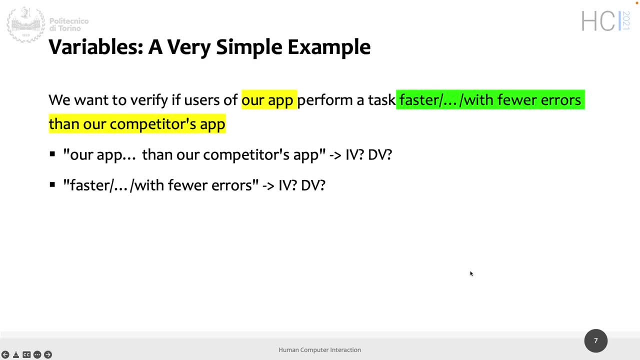 and dependent variables. So nothing so distant from the thing that we imagine like here. We want to verify if the user of our app performs a task, a specific task, faster, let's say, than another application. So something measurable, something that contains both the independent and dependent variable. 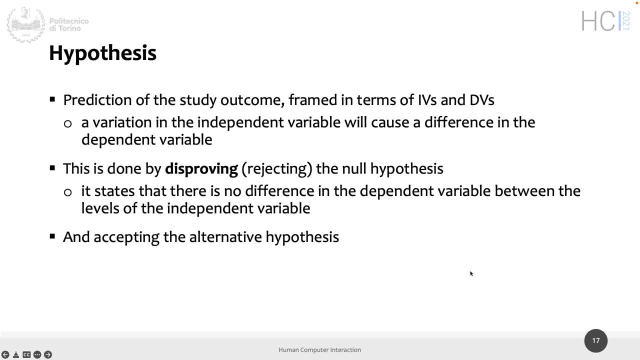 But What we want to do is not verifying an hypothesis. We want to disprove or reject the null hypothesis. So, while our hypothesis will say that we want that version 1 of our application is better or is faster or create more engagement or generate less errors than version 2, and 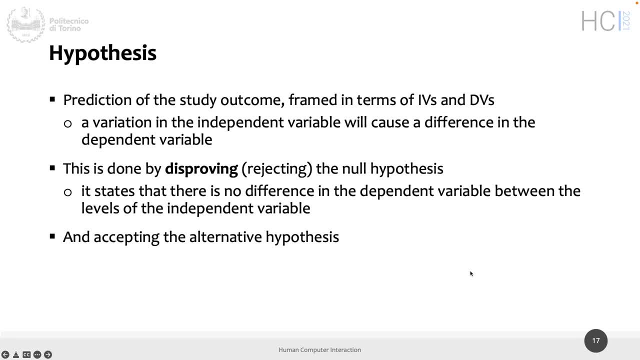 we need to measure in a specific way: fewer errors, what means more engagement, what means what we can measure. we use statistical tests not to confirm that hypothesis but to disprove, let's say, the overall hypothesis. So let's say we want to do a statistical test. 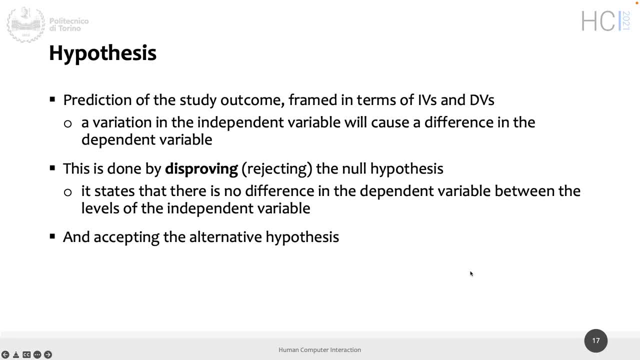 Hence we are doing a statistical test. How do we verify that algum solvency prevails in relation to the nepal and arman? How do we work with proper optimization of these variables so that print is more efficient than genere MMA and對啊 X in the 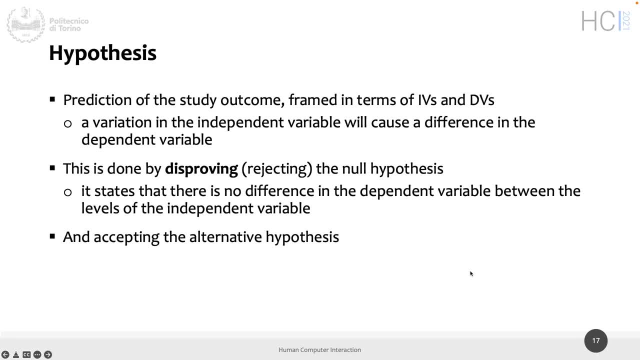 version 1, Where, even if your insertion code is runner, how will that save you? Let's say the opposite of this hypothesis, That is called the null hypothesis. Why does the hypothesis say that a variation in the dependent variable will close will cause a difference in the dependent variable? 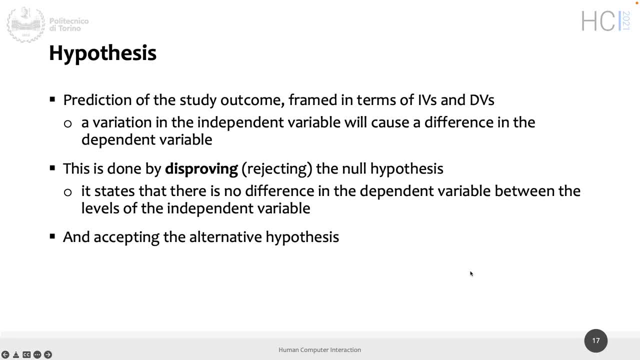 Version one is better in some way than version 2.. The null hypothesis says that there is no difference in the dependent variable between version 1, which calls for integration into theControl保alt and depositable, and version 2.. So the null hypothesis states: 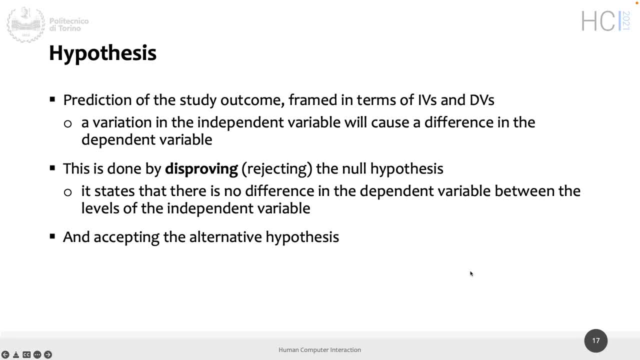 that the difference that we want to have in terms of dependent and independent variables does not exist. There is no difference. So we want to work with the null hypothesis, to in a way, enact the null hypothesis with. our goal is not to confirm the null hypothesis, because it will say that 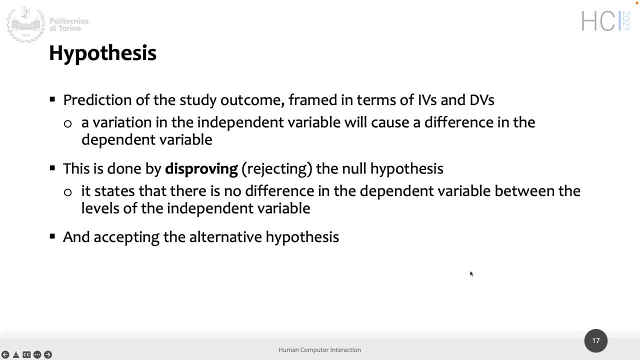 the two versions will not be different. So our goal is not really met, but that we want to disprove that hypothesis. We want to say that there is a difference. So we want to reject the null hypothesis, thus accepting our original goal, our original hypothesis. 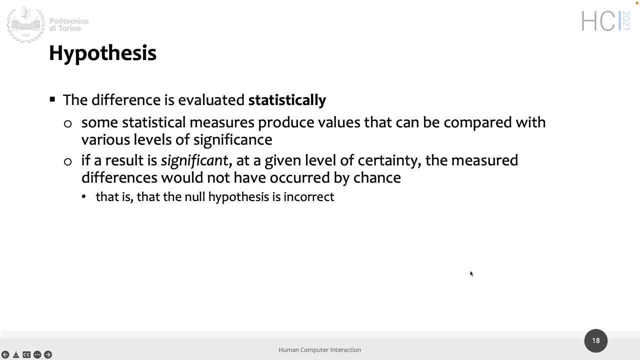 And this difference why we work with null hypothesis, because this no difference is evaluating that statistically. So we will have some statistical measure that can produce results according to some level of significance And so we can say at a certain point that the result is significant, is statistically significant. 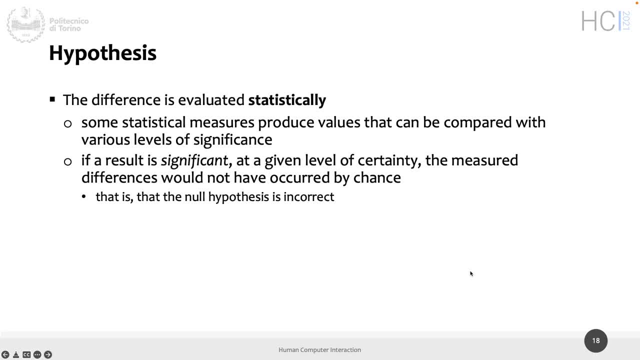 So the measured difference, the difference that we notice, cannot be accorded by chance. It cannot be occurred by chance. It cannot be occurred by chance. It cannot be occurred by chance. It's not by chance that we have this difference, But it's probably if we generate, if we redo the experiment. 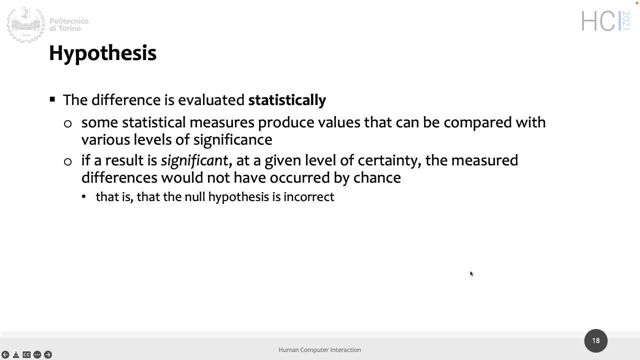 with the same null hypothesis, we'll get comparable results in a certain degree of interval, So let's say 95%. if we repeat, we will get the same results, similar results in the same way, for 95% of the time. 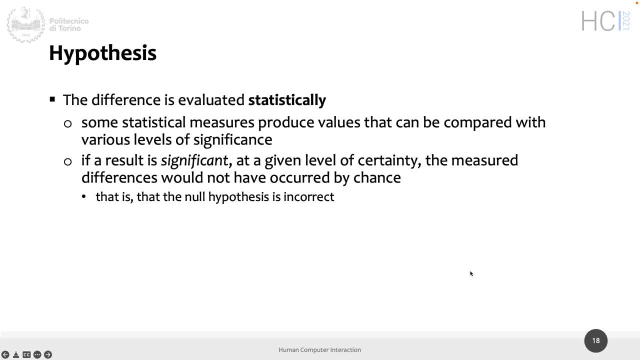 So we can say: That is, that will again. will not happen by chance, But it will be. if we replicate that, we are quite confident that we will see the same difference, Maybe not exactly the same number, but we will say: 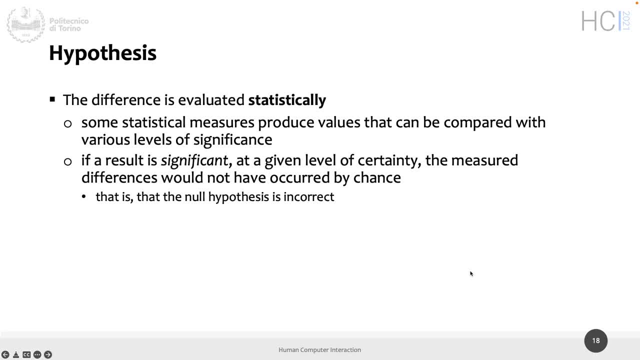 that still, version one is better in some way than version two, And we do this again by saying that the two version, the levels or the independent variable, have no difference. According to the dependent variable, the things that we are measuring on, 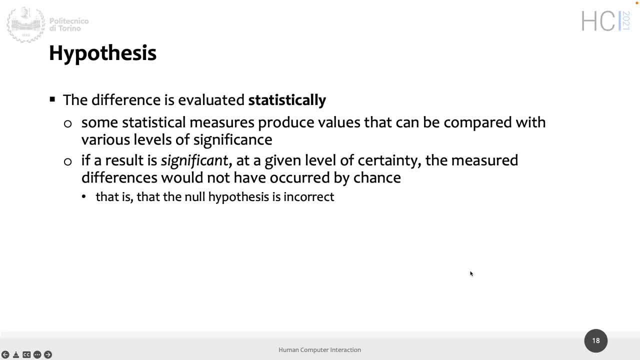 So if there is instead of difference, we can reject the null hypothesis, We can say the null hypothesis is incorrect And then, as a consequence, accept the null hypothesis. If this is not the case, we cannot say: pay attention on this. if this is, if we notice. 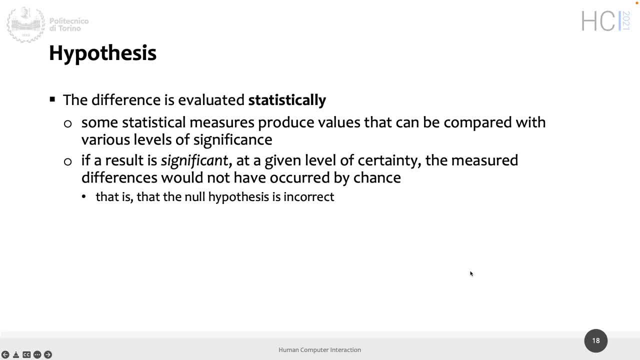 a difference, we can say: the null hypothesis is disproved and we accept the alternative hypothesis. That was our goal. If we cannot see a difference, we cannot say: oh well, so we there is actually no difference and we reject our hypothesis. 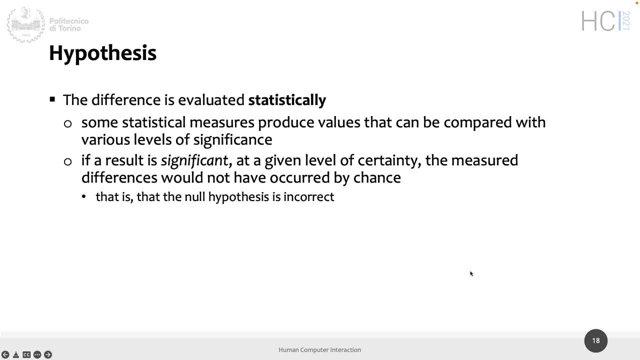 What we can say is: we don't know. So the null hypothesis cannot be rejected, It cannot be disproved, And we don't know if there is actually a difference or not. The idea in this controlled experiment, the idea in this statistical task analysis, that 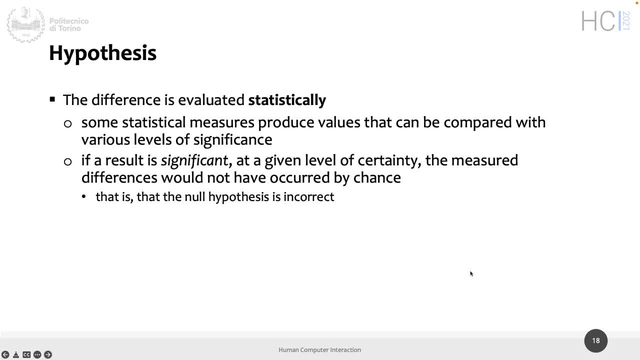 we can have is always to try to reject the no difference. And then if we can reject the no difference, then it's good And we can say, yes, there is a difference. But if we cannot, We cannot say there is no difference. 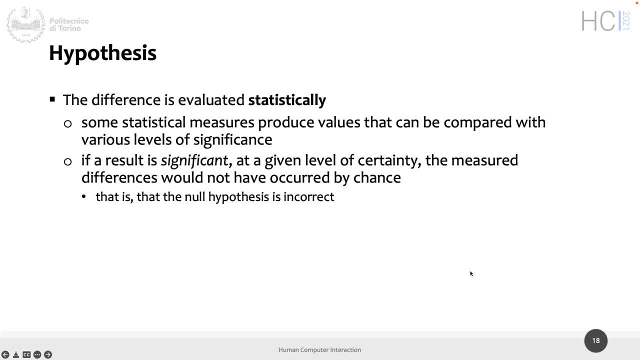 We can just say we don't know. We should probably run a larger experiment or pick other type of people or pick up other measure to see if there is a difference. But this is central. We cannot say we approve the null hypothesis and so there is no difference. 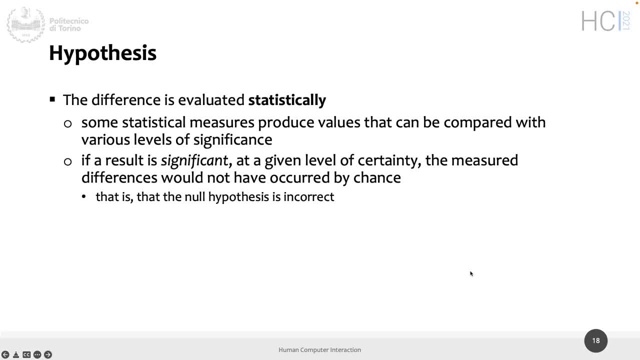 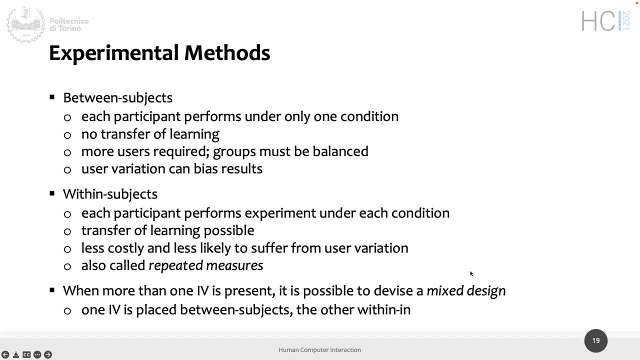 This is something that statistical test doesn't tell us anything about this. So, defining a hypothesis, we can say, let's say, version 1 of our application. our hypothesis, our alternative hypothesis, is: version 1 of our application is faster than version 2.. 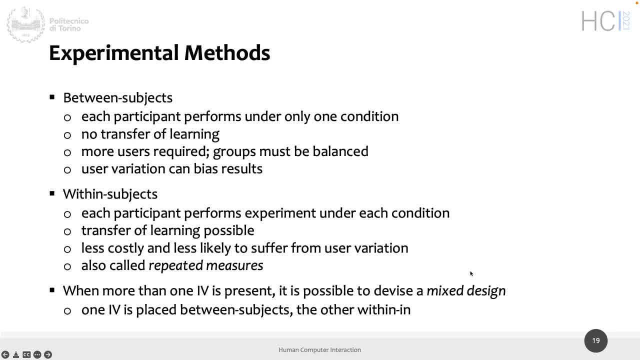 This is our alternative hypothesis, What we want to have: Version 1 faster than version 2.. The null hypothesis in this case will be that there is no difference in speed between version 1 and version 2.. And we are going to make an experiment: measuring time, measuring speed in a way to demonstrate. 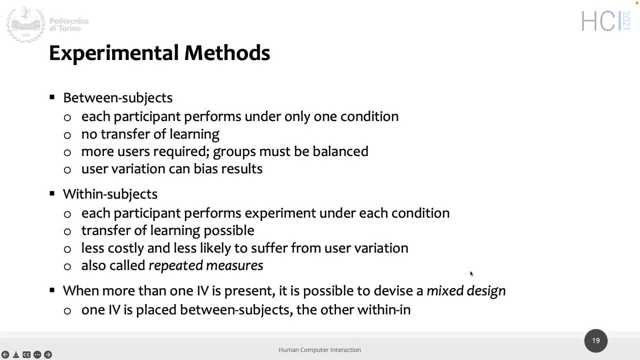 that that hypothesis is false. And if we can, we can say okay, so we can accept the null hypothesis, The other hypothesis, the alternative hypothesis, And so this is framing in hypothesis, framing in dependent variables, with levels, et cetera. 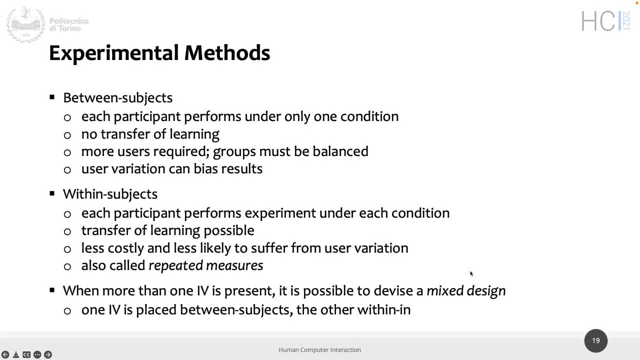 Another component of a control experiment that we have to decide is how do we run the study. Last time we have seen we have taken, for exemplifying the independent variable levels, a linear approach. We said participant number 1 will get all the values. 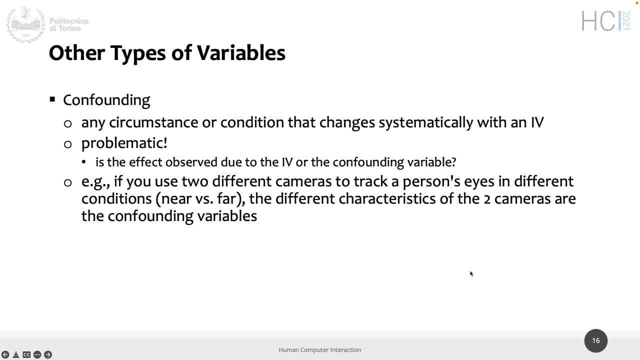 And then the participant number 2 will get all the values, And then the participant number 3 will get all the values, And then the participant number 4 will get all the values, And then the participant number 5 will get all. Let me see if there is still here. 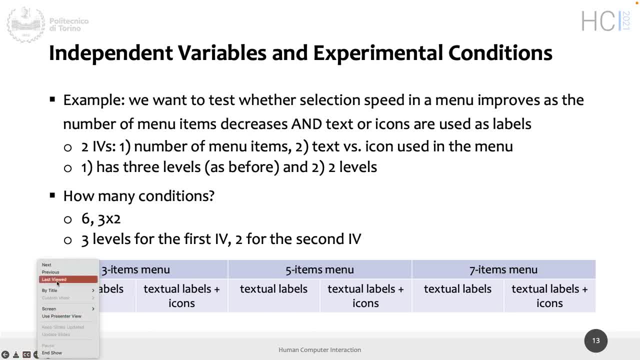 We'll get all these, All these in order. So first the three menu item with the text label, Then the three menu item with the text label, with icons, Then the five menu item with the text label, in order. So participant 1 will get this thing. 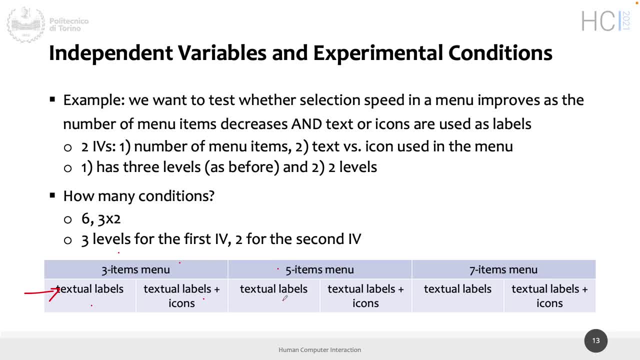 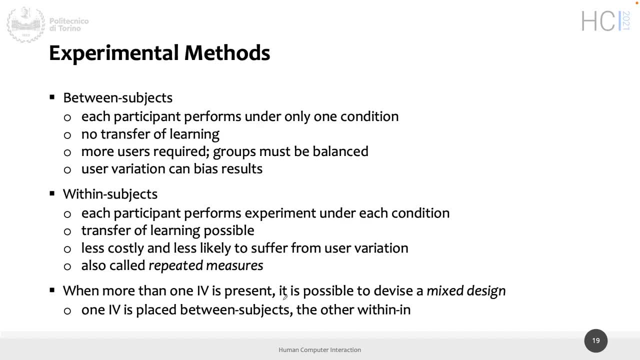 Participant 2 will get all the conditions in order from the first one to the last one, And this is one way to conduct the study. That is called within-subject, So remember the subject means participants, So within-participants. 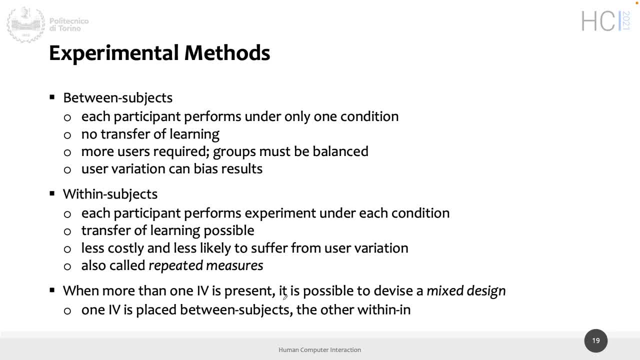 Which the idea of within-subject is that each participant performs the experiment under each condition. So participant number one will get the three item menu with the two icons versus non-icons, Then the five, So one participant will see everything, All the conditions And. 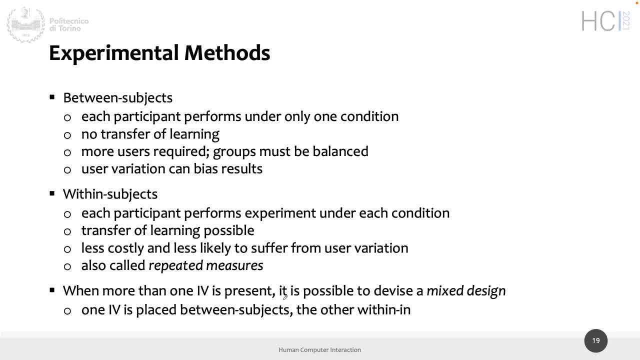 other participant again. The other way is what is called between-subject. Between-subject means that each participant just perform and see one condition, Not all. Just one, Just the three menu item, And another participant will see just the five menu item. 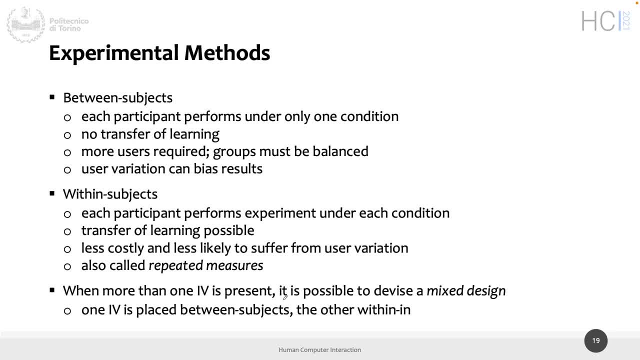 And another participant will see just the seventh menu item. One participant will see just one condition And then after the task in that condition, goodbye, Get another participant. So these are clearly advantages and disadvantages, Right? So, as you can imagine, if you have just 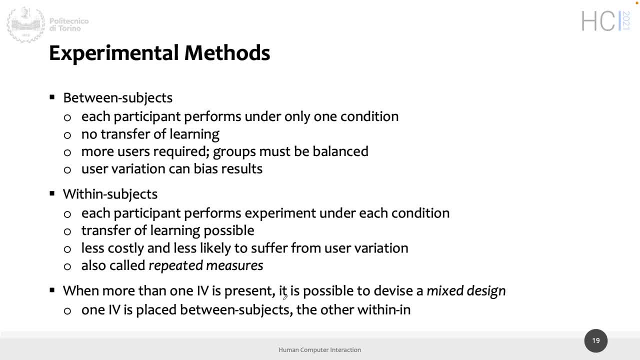 three conditions. let's say the menu three, five and seven menu with the same task with within-subject. if you have three participants, you have data three time. let's say three piece of information about the three menu item. three piece of. 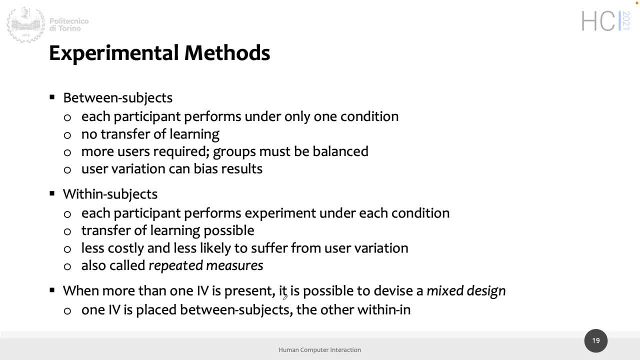 information about the five menu item and three piece of information about the seventh menu item. Because everybody do everything In the between-subject. you will have one piece of information about the three menu item, One about the five and one about the seventh. So you have three time less data in the dependent. 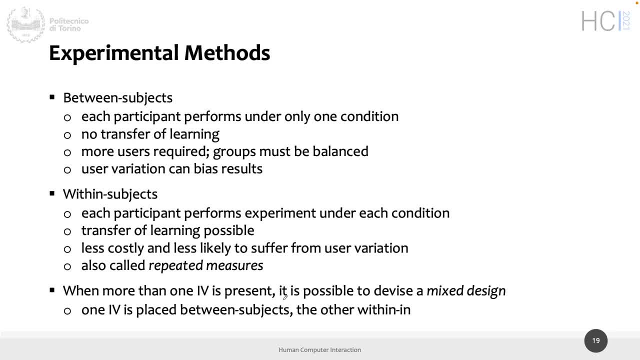 variable. So a first disadvantage of between-subject is that you need much more people than the within-subject Because, again, within-subject you have three participants doing everything, so you collect information about everything. With the between-subject you need, if you want, the same amount of. 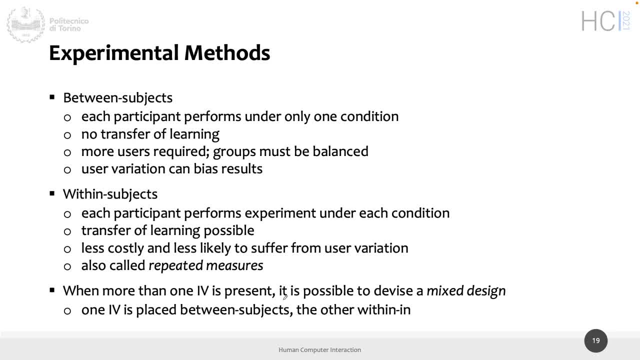 information. you need three time the participants if you have three levels in the menu To have the same amount of information collected- data Because each participant performs just one condition. So this is clearly a disadvantage And also you need in between-subject. 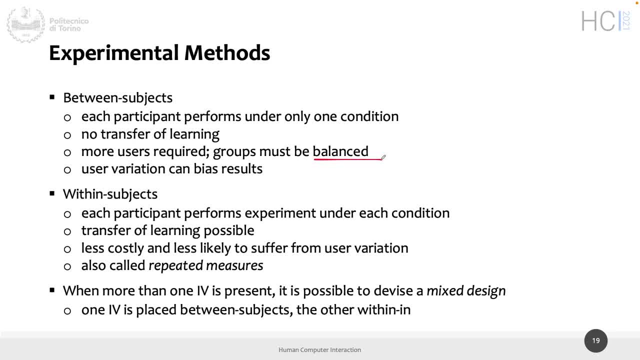 balanced groups. So if you have five people in the three menu item, another five in the five menu item and another five in the other condition, you will need more or less the same population. You cannot have young people in the first condition and elderly. 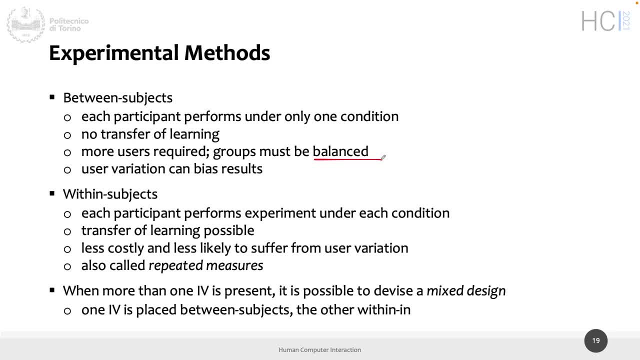 people in the second, Because then they are not going to be comparable. You cannot have expert in the first and not expert at all in the second. Because, again, you want to compare this information, the data that you collect, So it should be homogeneous, And this doesn't. 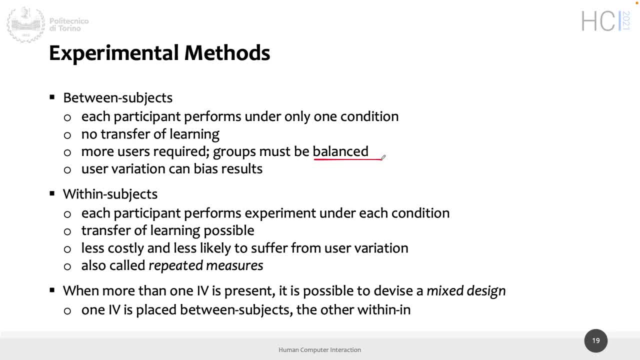 happen in the between-subject because you have the same people doing everything. So you have naturally balanced the group. You have just one group that do everything. Conversely, 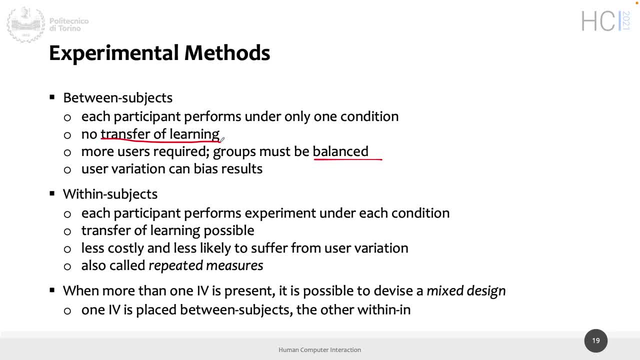 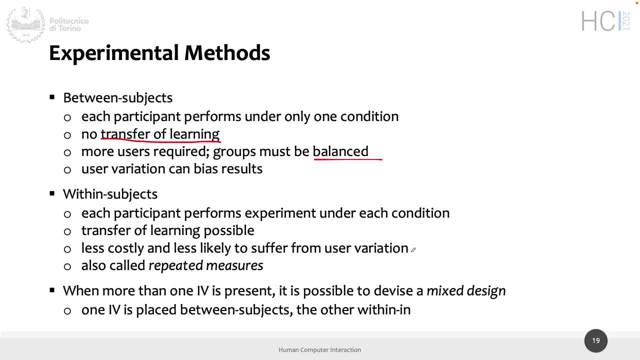 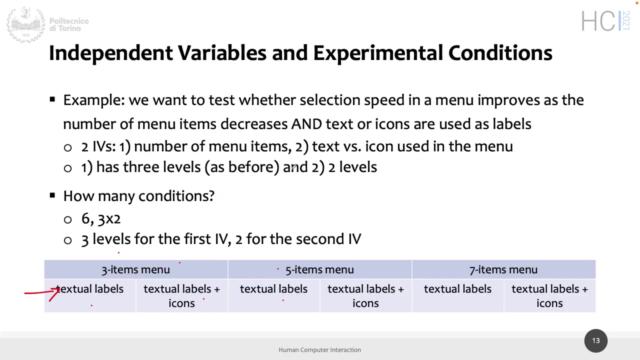 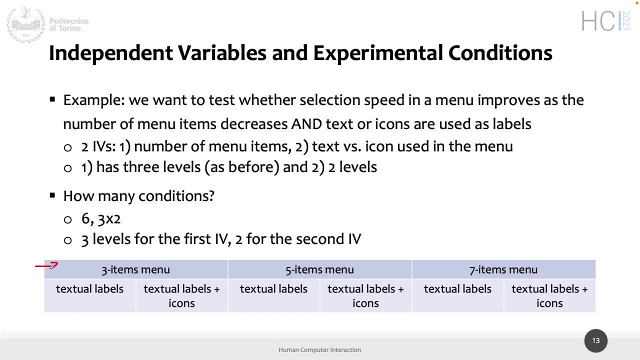 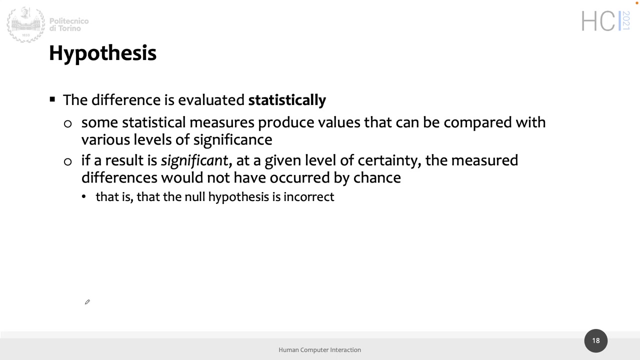 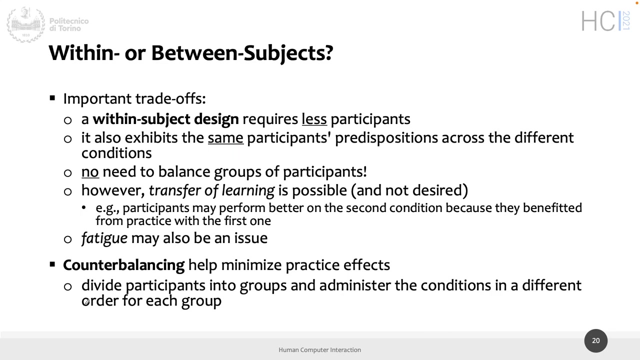 can have fatigue at a certain point for the participants because it's very lengthy. it's very long also the study and you cannot do really anything about. 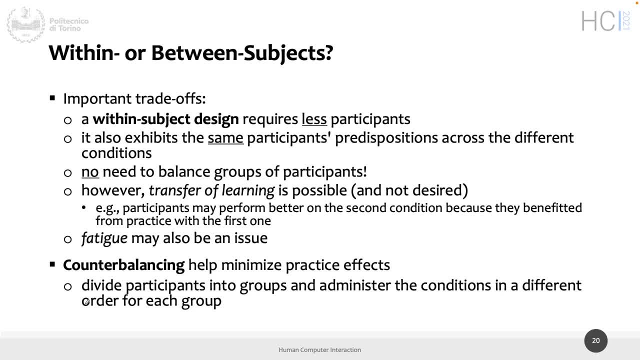 fatigue. maybe you can have a break, but not a lot, so you cannot really fix that. but you can try to minimize the transfer of learning. that that could be done. not eliminate at all, but minimizing. yes, you can minimize the transfer of learning. how doing what is called counterbalancing? you counterbalance participants among 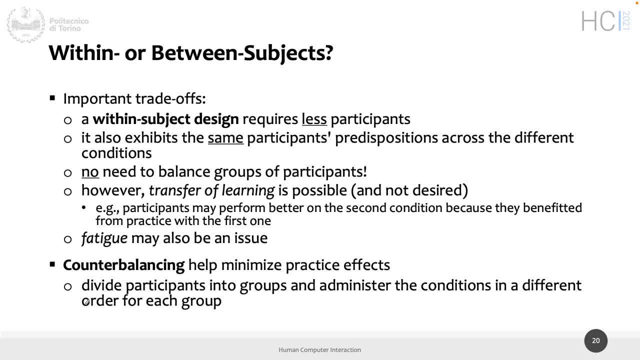 the condition. so you divide in a way your head participants in two groups, in groups and give the condition in a different order. so participant number one will get the condition in the order one, two, three, four, five. participant number two will get the condition in the order five, four, three, two. one. participant number three. 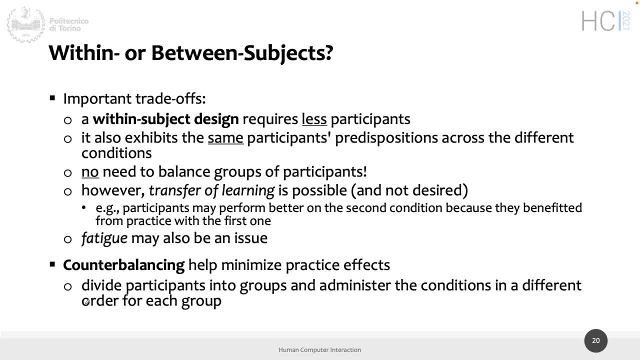 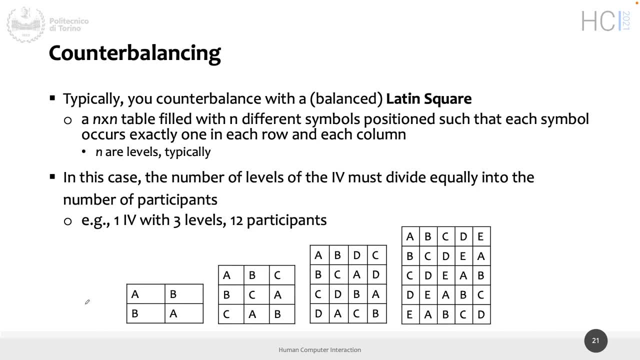 will get the condition in the order: one, three, five, two, four, etc. so you make things in a different order to counterbalance the order. so this is not random counterbalancing. you can also do randomly, but it's proved the counter balancing work well for transfer of. 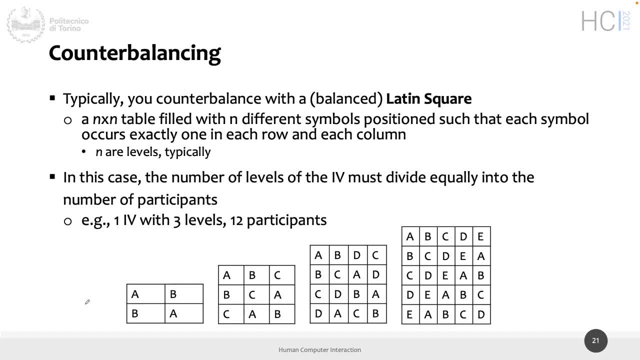 learning. so for reducing transfer of learning, if you use a balanced Latin square. what is the Latin square? a Latin square is a table and for N where n are levels. so if you just have two levels for an independent variable, it will be to be a two per two table in which you have a. 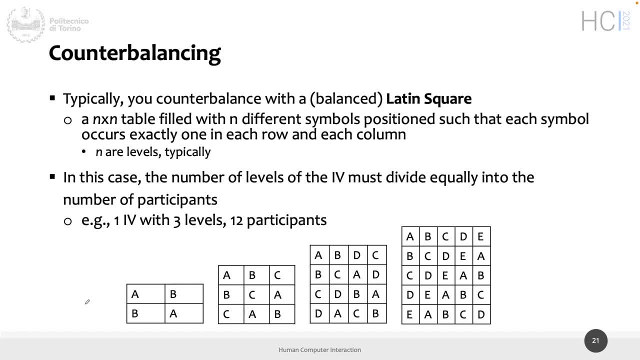 different symbol for each row of each column and each symbol is the condition. So here you have condition number one and condition number two, A, B, And then you have condition number two for another participants and condition number one. So if you have two participants, you have, you can use this. 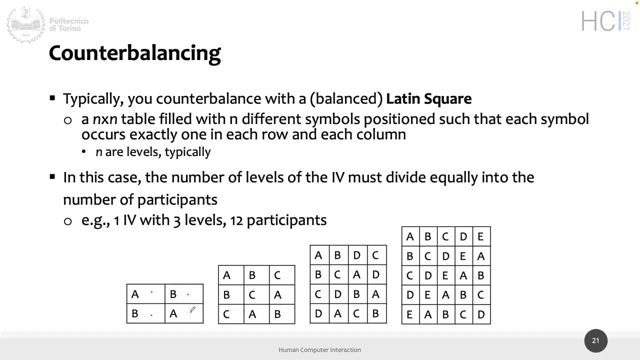 One participants will do condition A and then condition B, and the other participants will do condition B and then condition A. If you have four participants, you can still use this. Participant number one and participant number two will do condition A and then condition B, And participant three or 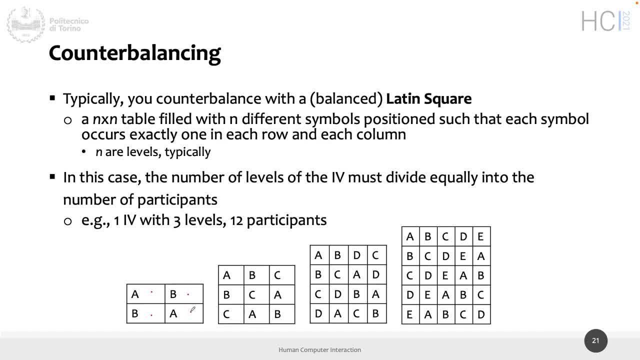 four will do condition B and then condition A. So this is not between the participants, not constrained by the participant number, but the levels of an independent variable. So that's why, before I told you, you divide your participants in groups, Because here, 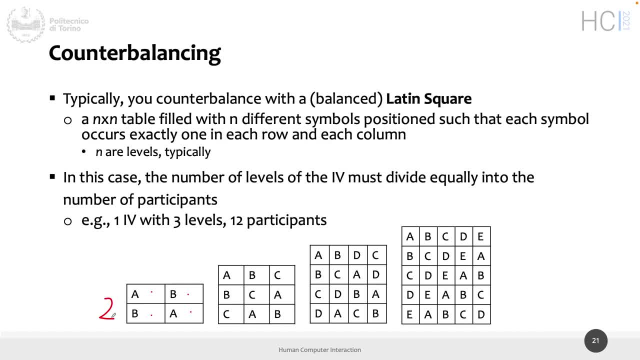 you can only have two groups. So if you have two participants, it is one group per one participants per group. If you have four, it's two people. If you have 20 people, 40 people, you just have two big groups: ten-ten, twenty-twenty. 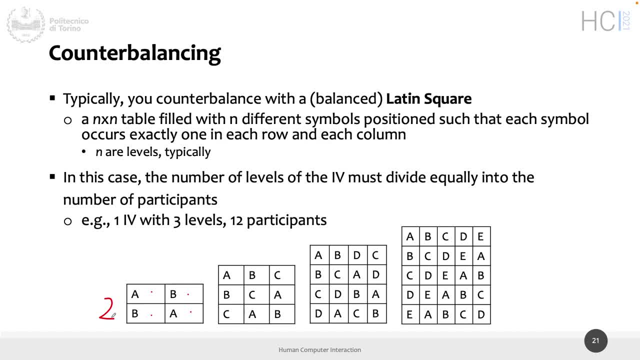 etc. A balanced Latin square is, however, not just split in that way, but as a rule, and the rule say that each symbols must occur exactly once for each row and column. So here that is a simple case: A happened just once in the row and in the column There is no. 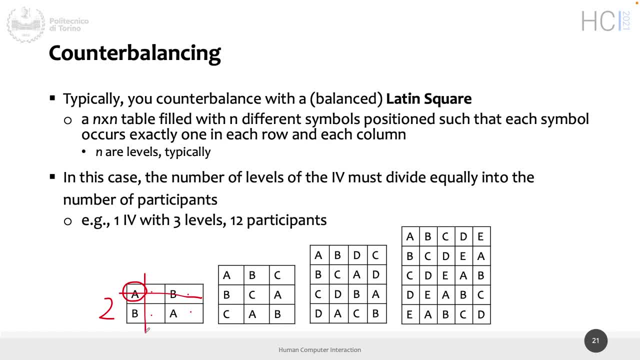 other A here or here, And same things for B, And so here it's very simple, you just have to level. here is a little bit more tricky, clearly, Because you have more number, but even here A should appear once in each row and in each column In. 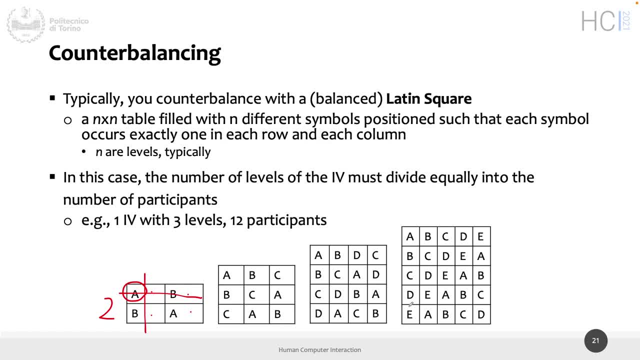 this case, if you counterbalance in a within subject experiment, you must divide equally the participants according to the number of levels. So if you have three levels, one dependent variable, with three levels, you should have, for instance, 12 participants, Because 12 is. 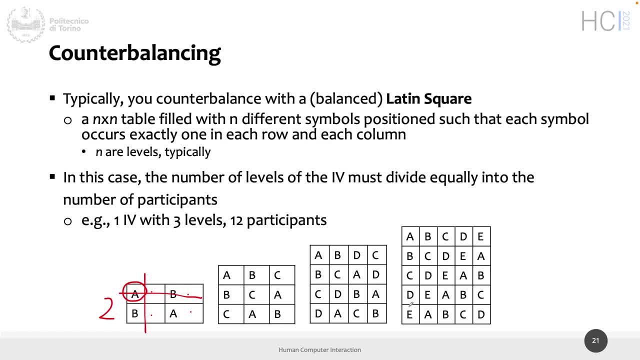 fully divisible. you can divide 12 by 3.. Also by 4,, if you want. You cannot yet have 11 participants because you will have three groups. let's say different, Because 11 by 3 is not an entire number. 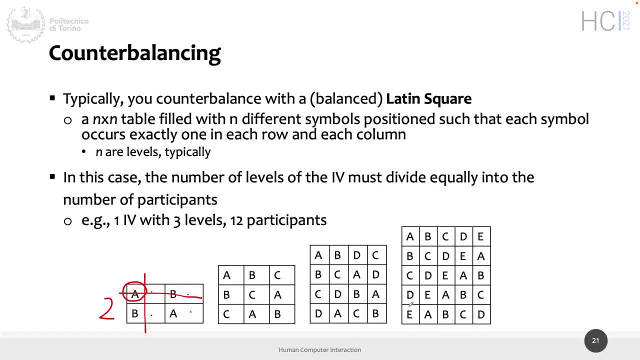 You have some rest. So with three levels you can have three participants. that are too few. We said at least 10.. So 9 we could also have, but still less than 10. So you can have 12. You can have 15.. You can have a number that is created by three. 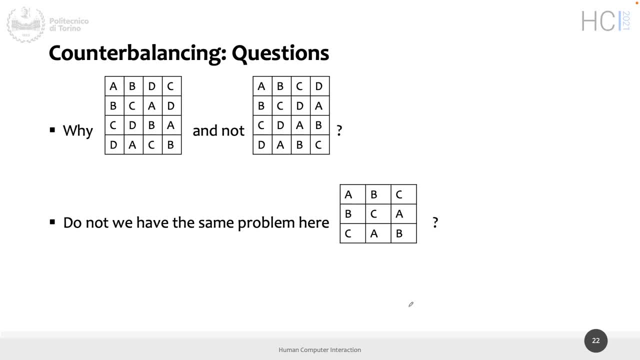 So this is a balanced Latin square. So look at this. the first two In which we have this is four to four. Both are Latin squares, So they both respect the rule. So A appears only here, B appears only here, C appears only here in. 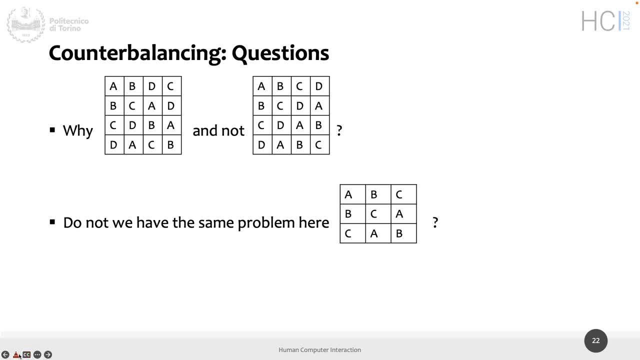 the row and the column. And same thing for D And same thing here. A appears only here, B appears only here, D appears only here and C appears only here. But if you look in the previous slides for the 4 to 4, you don't have the ABCD version, You have the ABDC. 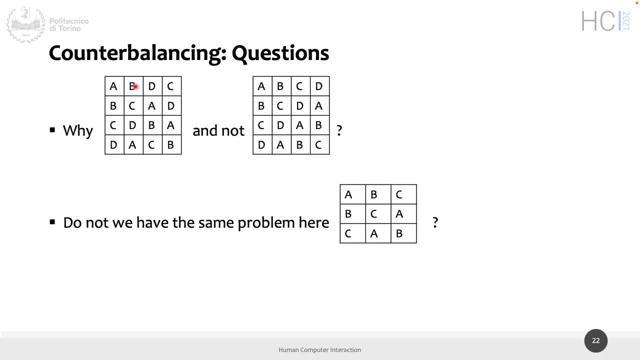 version. So, given that both are valid Latin square, balanced Latin square, because there are 2 per 2,, 4 per 4,, 3 per 3, so they're balanced that way, why the first one is better than the second one? 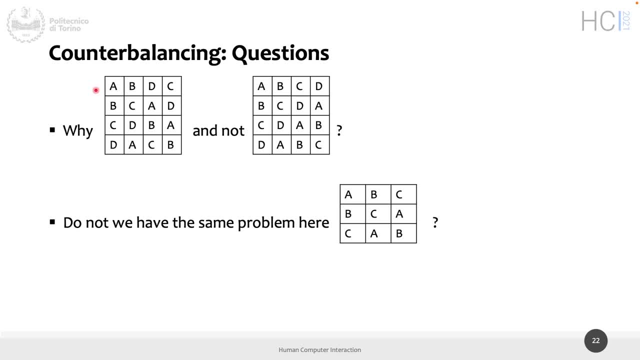 It still has to do with learning effect. Repeat: Yes, Yes, you have these. It's right, You don't always – it's not always ABCD, but yes, you have chains. You have B and C that comes together here and also here. and 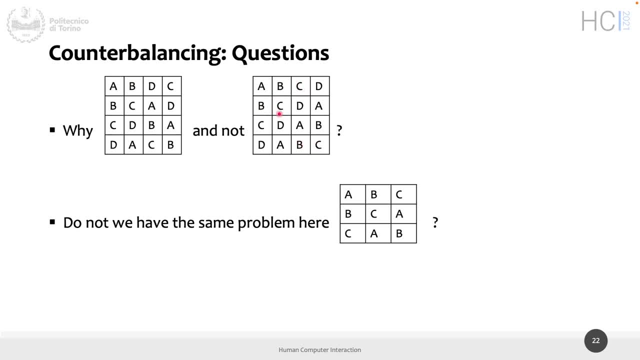 also here, and the same things for C and D. So you solved the longer learning to transfer, but you still have smaller learning to transfer. And so notice, here, here these things doesn't happen. So here let's pick B, Here after B, you have a D, Here you have a C, Here you have an A And here you have 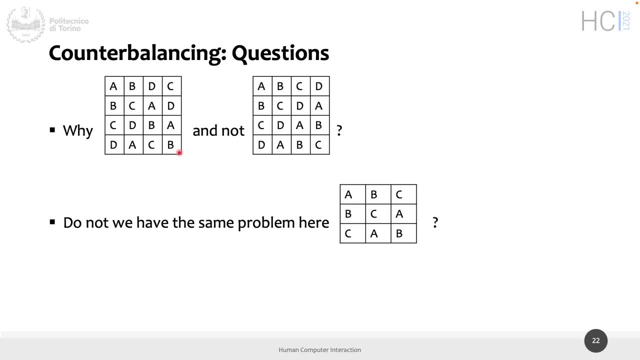 nothing And the same things apply to everything. So the first one is better than the second one, because you don't have this relationship, this repetition, this pattern. So you have this problem with big, like 4x4 tables. You don't have this. 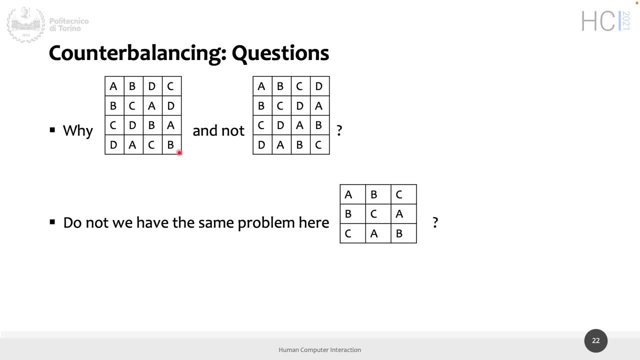 problem with 2x2,, clearly, because you just have two levels, It's easy, But you can have also this problem. So one way it could be: let's start with A, B, C, D, and then you have to move things in a way that you don't have a C. 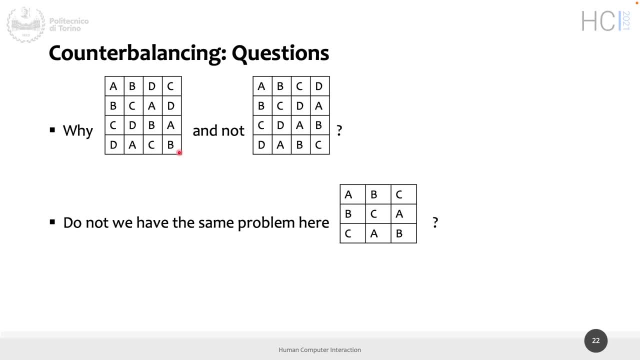 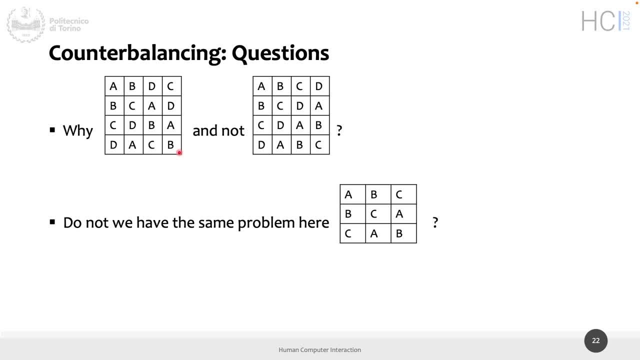 following an A more than once, et cetera. So this is one way to do it. It's not the only way. So still a Latin square. both are Latin square, both are balanced, but the first one is better than the second. 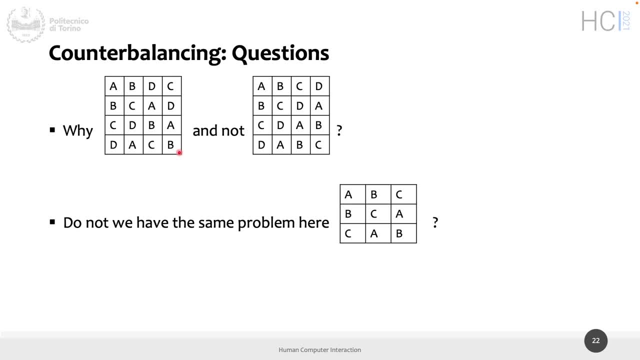 And we don't have the same problem in the other three-per-three table. Do we have the same problem in that table? Yes, no. Who say yes? Who say no? You say I don't know? okay, Yes, we have. 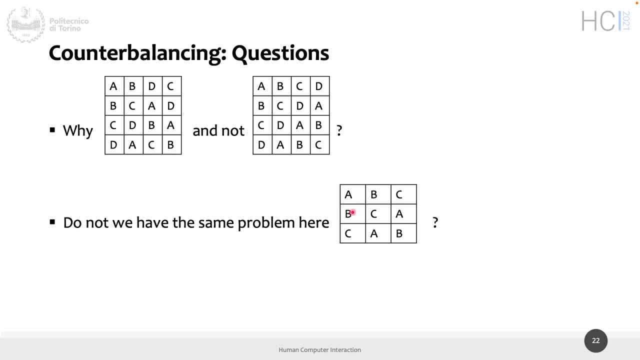 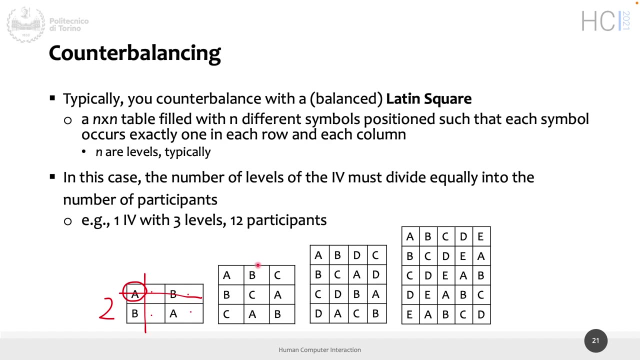 B and C, B and C. That is probably the only pattern in this three-per-three, But here in this table I put this one. You have also the problem here: B, C, B, C, D, et cetera. 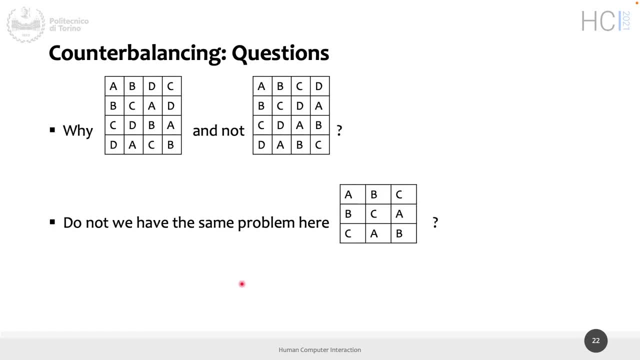 So this is the table that you're going to use. I put that here Why. I mean, there is this pattern. How can we solve it if we want? So one thing is to say there is this pattern, It's fine. 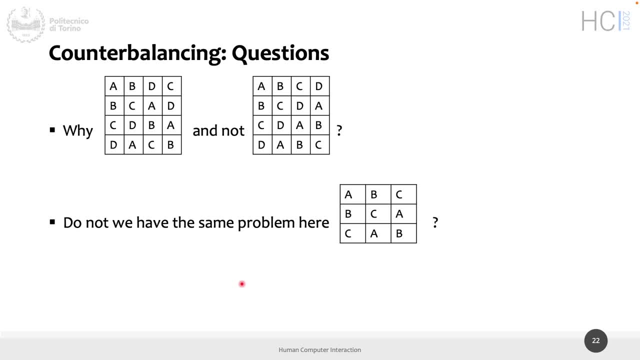 We recognize that there is this pattern And that could affect results. So in the four-per-four table it's easier to fix. In the three-per-three, five-per-five it's a little bit more tricky to fix it in a Latin square. 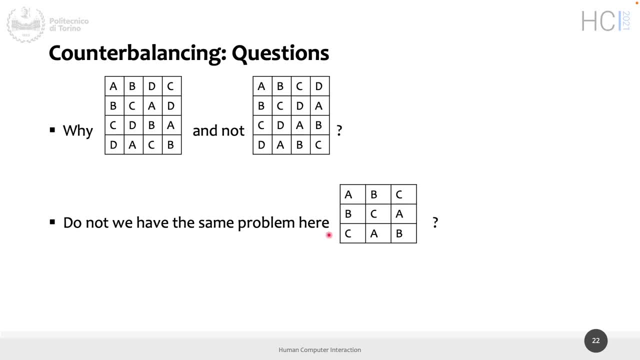 So we can either say, okay, accept that there will be this pattern, So maybe there will be in the results some transfer of learning between B and C. So I clearly acknowledge that there is And the alternative that we can have, how can we change? 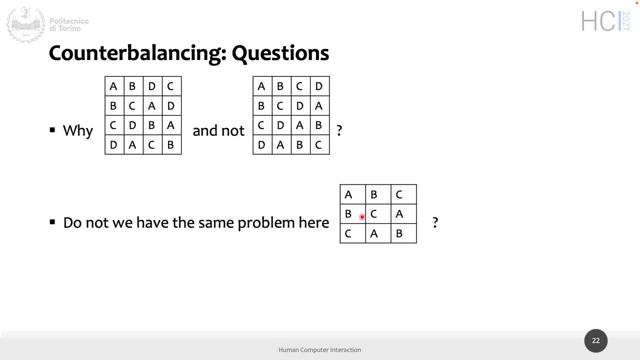 How can we create a table for avoiding this problem? We can't- is not totally true. We can't have, we cannot have a Latin square three-per-three avoiding this problem. That is true. We should have a bigger table If we, for instance, 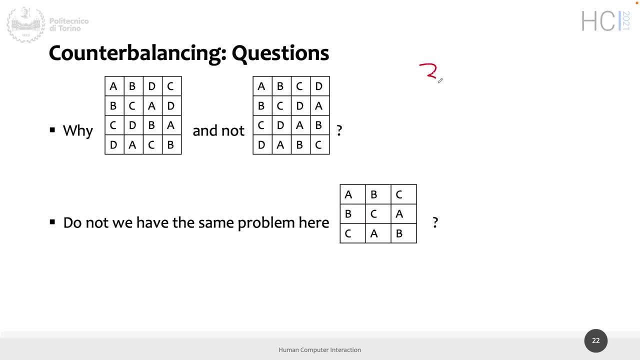 build a- I'm not going to build, but a three-factorial table. we can avoid this problem. Clearly it will not be a three-per-three table. It will be a much bigger table as a number of elements, But with that. 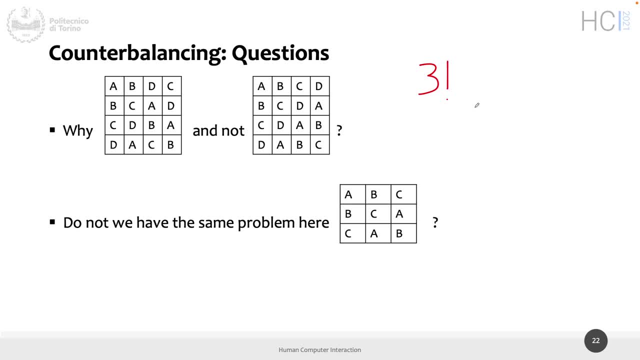 we can avoid this problem, But we need probably more participants, Because here we need, let's say, 12 participants With a three-factorial. we need and we'll have: with 12 participants, we'll have three. 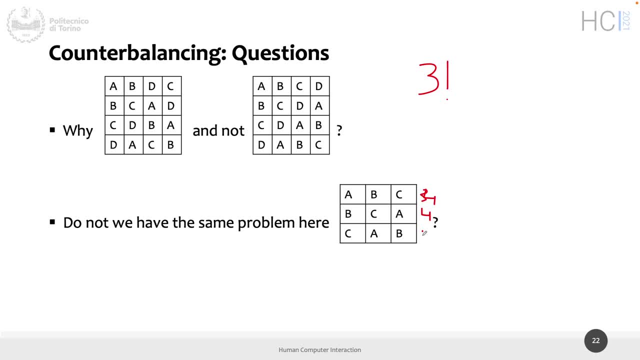 no, four here, four here and four here. With a three-factorial with 12 participants, we will not have four participants for each, let's say, row of the table. So we need, we need, we need. 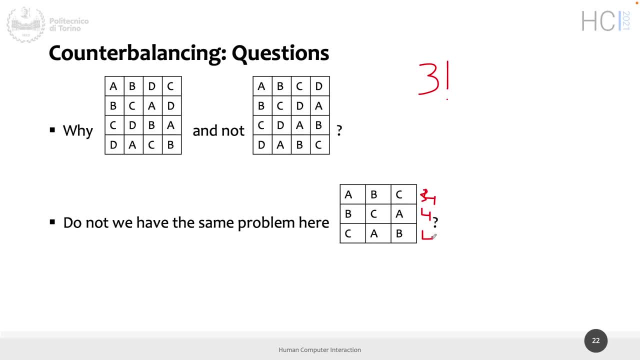 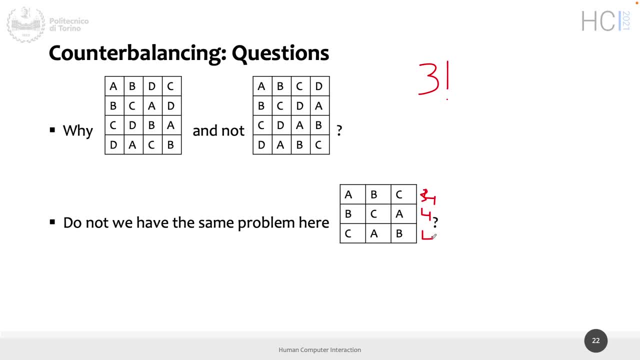 a table built with a factorial number of row and scholar which sells Otherwise. we can acknowledge that there is this pattern and consider that when we make some assumption or experiment, If we have not as well a three-per-three table or a five-per-five, 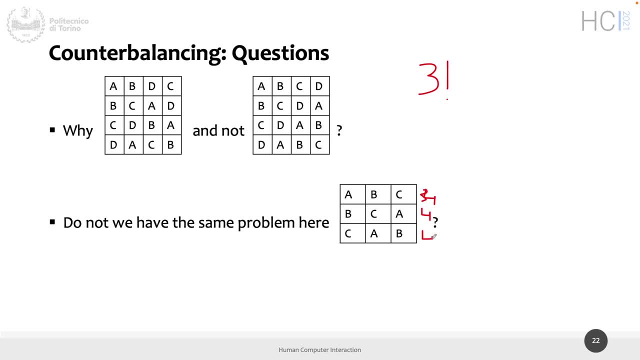 so if we have we have four levels is not a problem, because we are in the other case, or six levels is not a problem, And for levels here we can also mix if we do everything in a within subject. 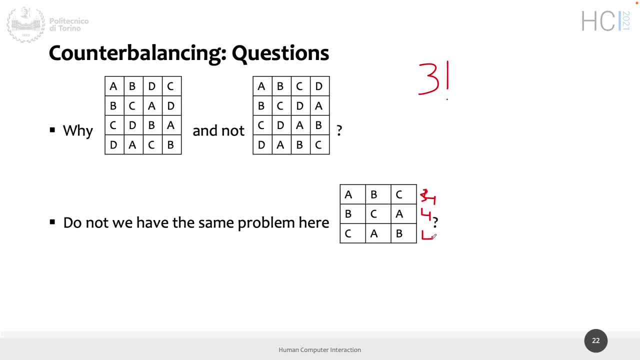 we can also have multiple independent variables, And so we can have six levels, meaning maybe one, let's say one level for the first independent variable and two levels for the second one. So three and three. so two levels and three, Two levels, two. 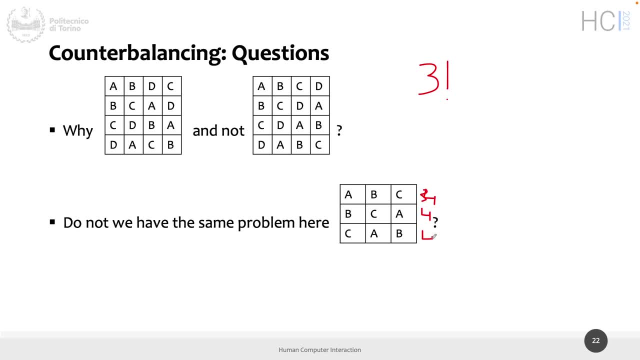 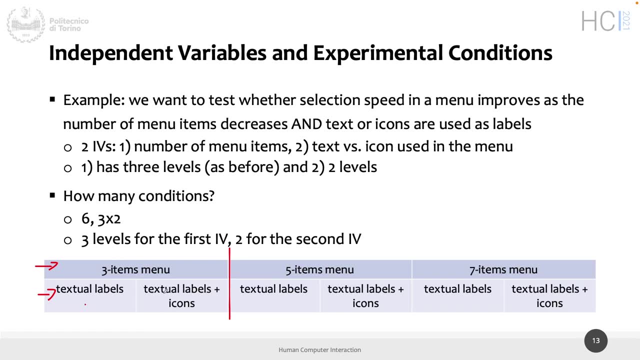 Two and two. Okay, you got it, So you can also mix. So here we have. if we do everything within subject, we have one, two, three. We can consider these as condition A, these as condition B, these as condition C, et cetera. 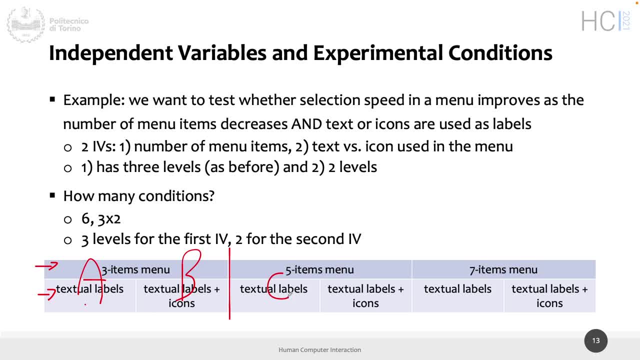 So putting together three item or five item, So three item with the text and five item with the text, et cetera, If we do everything within subject. So in this case we have six condition with levels, even if there are two independent variable. 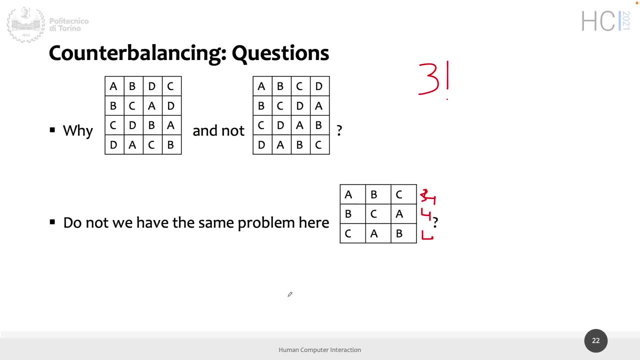 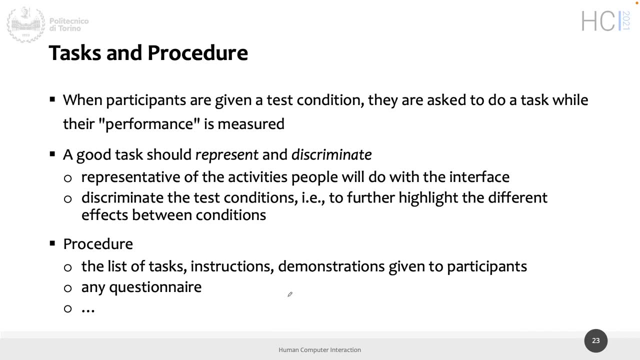 Okay, and this is how to minimize learning effect. In some case we can just minimize a bit. We cannot solve everything in the learning effect Then we will have. so this is how to set up the study. Then we will have a task. 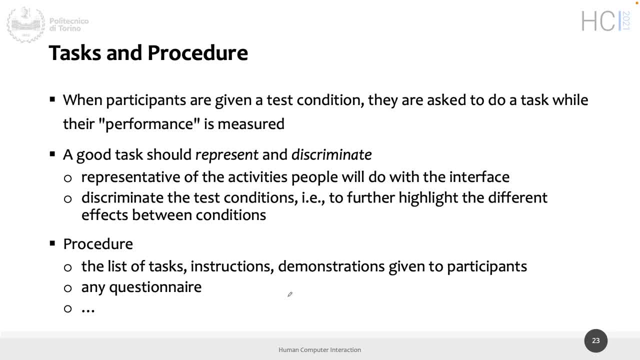 The task, that is, the things that we want to measure on, And tasks are similar to the task that we have seen in the past, With the difference that could also apply to the usability testing and the others, But here it's most important. 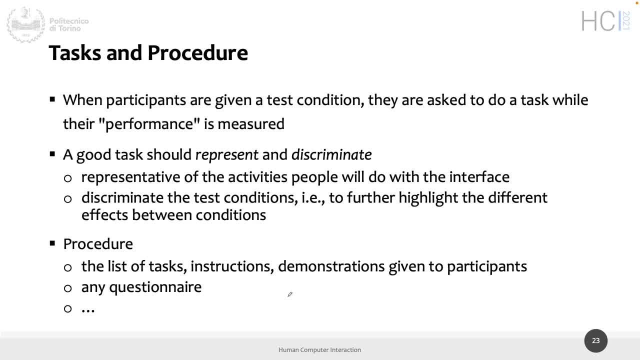 that the task both represent the action and discriminate the user. So in this case we have two tasks: The first one, we have the user. The second one: we have the user And the third one, we have the user. 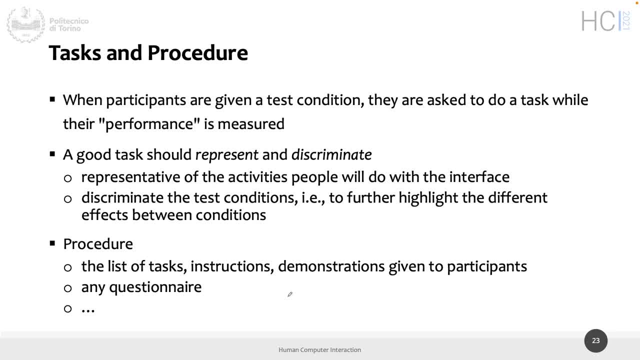 And the third one, we have the user. And the fourth one, we have the user. And the fifth one, we have the user. So the task should represent the action, So it should represent the activity that the people will do with the interface. 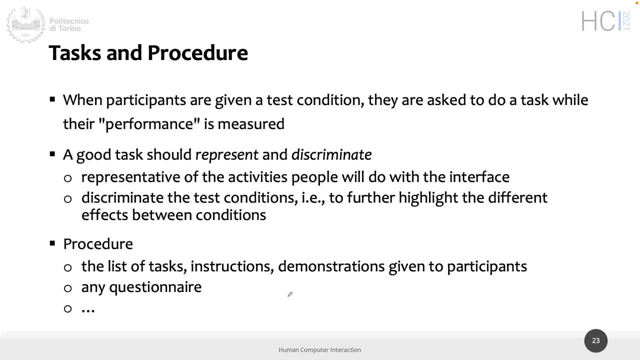 So click on the button, navigate the menu. So it should represent a realistic action that people normally will do, but also should be discriminative. So trying to further highlight the effects, the difference between the conditions, And as procedure, you will have the same kind of procedure that we already have for 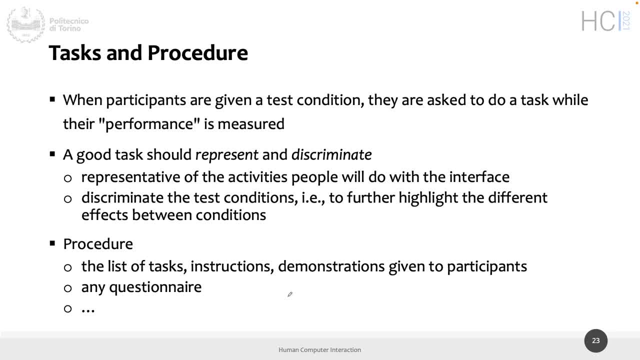 the usability testing. We need the list of tasks. We need the methodology within subject, between subject mixed. In the case of within subject, we will need the Latin square, the order of how the task will be given to the participants. 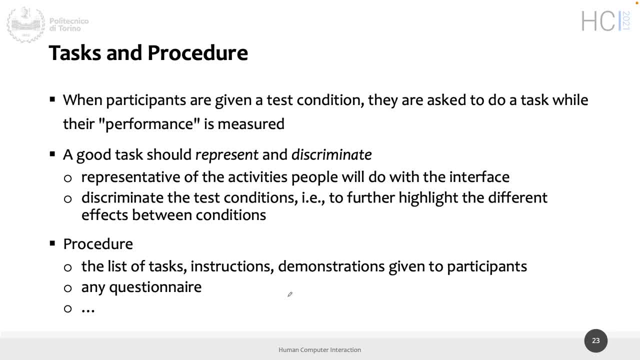 We need the target population, how many participants, how we recruit it, et cetera. We need instruction, the script, We need demonstrations. probably We also need a questionnaire: background questionnaire if we want additional information, Or screening questionnaire if we want to screen people before doing the study, to know. 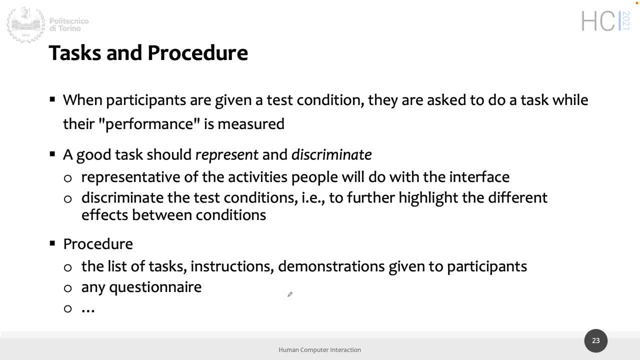 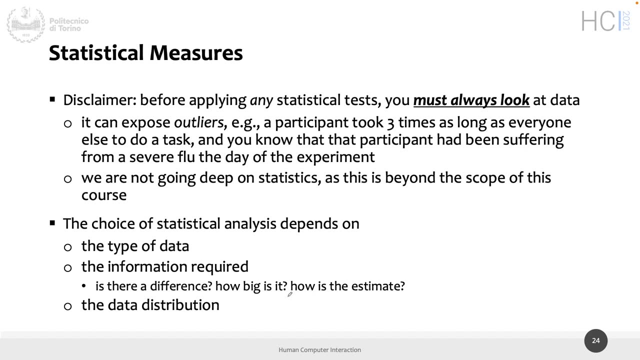 in which group. maybe we want to assign these people to keep the groups in case of between subject balance, Or to keep the overall group quite balanced, if possible. We need basically the same things that we need before, So that with all this information, we can run the task. 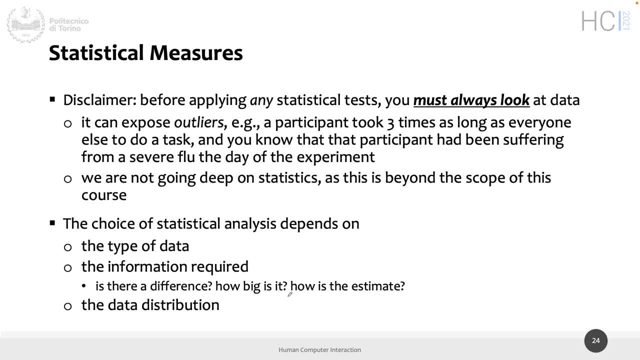 So let's imagine to have one interface that is simple case One interface in which we have a button that say I don't know login, or the same interface with the same button that doesn't say login but say learn more or any other text that 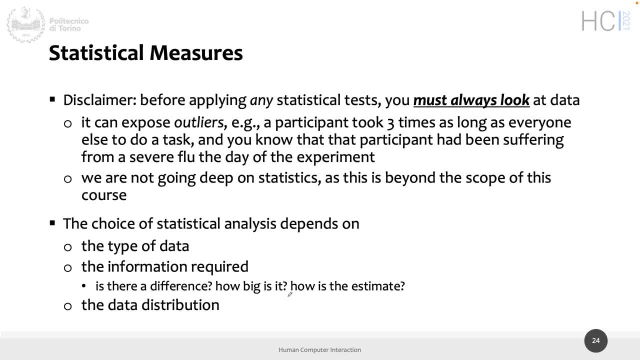 could be realistic And the task would be login on the interface or learn more about the application, Something that is significant and does not get the same text that is in the button clearly. So you run the test, You have 12 participants. 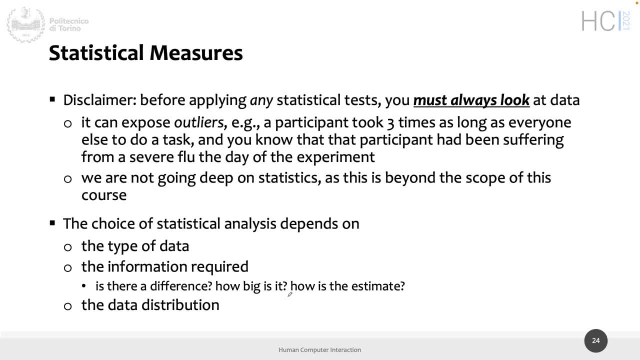 Or 100 participants. you do within experiment, mixed experiment, whatever, and you collect. So you're interested in the engagement. How many people will login or register? will click that button In the two conditions, In the learn more and in the login condition. 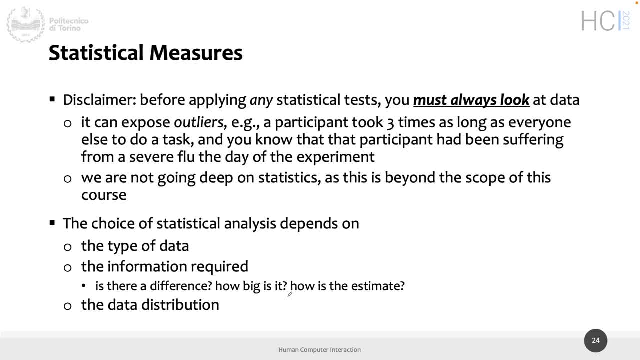 And you get some data. You get that out of your 12 participants. you will have- I don't know- eight people that click on login and four people that click on learn more, And this is a way to measure your engagement. So we said that this is hypothesis driven. 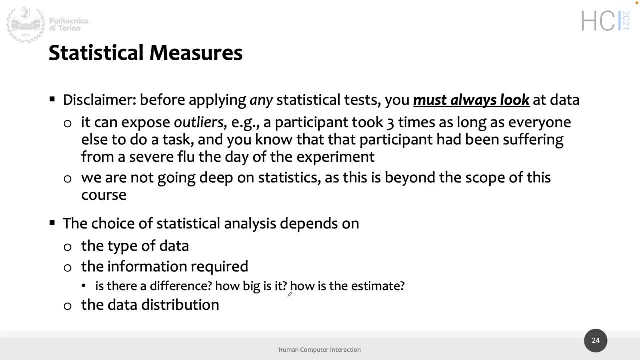 So we have an hypothesis that is, for instance, that the login button will generate more engagement than the other one, And we have eight people versus four, So it seems to have generated more engagement, But let's not forget that we have a null hypothesis. 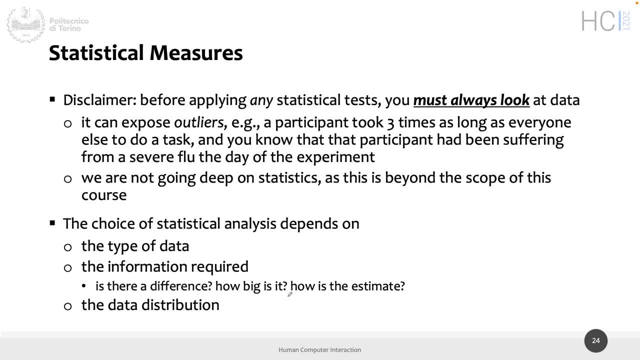 That is, that the two conditions will not have difference, So the same people will click on the button in the same way, No matter. basically the button present for the engagement. So we need to understand if these eight and four are really different or just happen by. 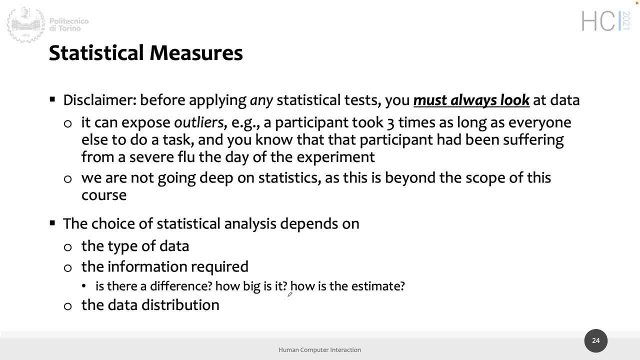 chance. So we get other 12 people. You will get more people clicking on the first one or more people clicking on the second. We will get consistent results or just a case that we get eight versus four. And to do that, to disprove the null hypothesis, we need to have some statistical measurement. 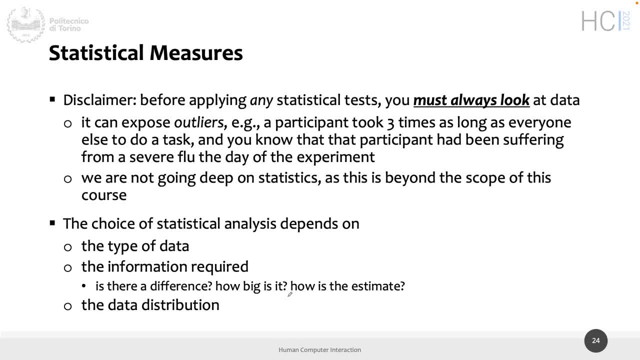 and statistical analysis. Some statistical analysis. That, as I said before last time, We are not going deep into that, so we'll keep at a theoretical level and we will see just one example of one statistical test to do one specific thing in a certain type of control experiment. that is easy. 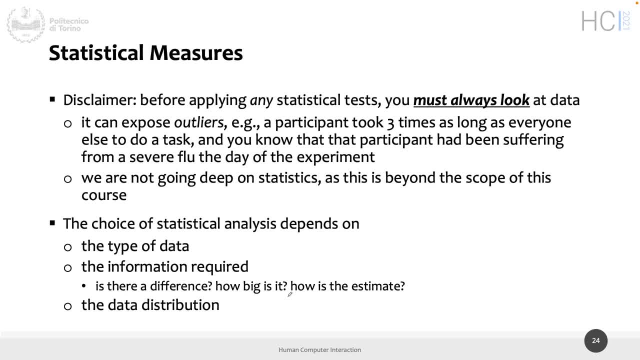 It can also be computed by hand. basically It's called the chi-square test. So you have this data and you want to apply some statistical test according to the number. There are some rules and we are going to say that. 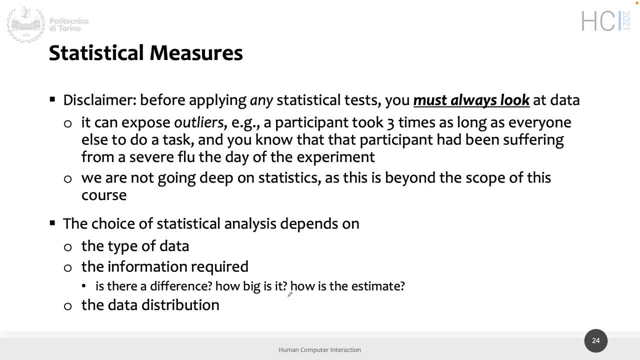 So the disclaimer here is: in any case, before applying any kind of statistical test, you have to look carefully at the data that you have To, for instance, look for outlier. So here there is an example of an outlier. 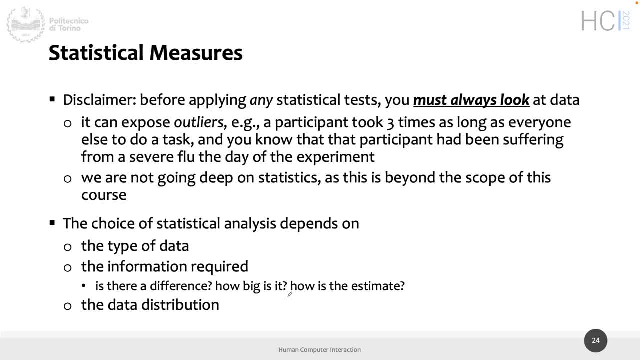 A possible outlier. So participants that took three times as long as anybody else to do a task And you know that that participant, for instance, was sick that day. The different experiments, So maybe all the time, were changed due to these participants. 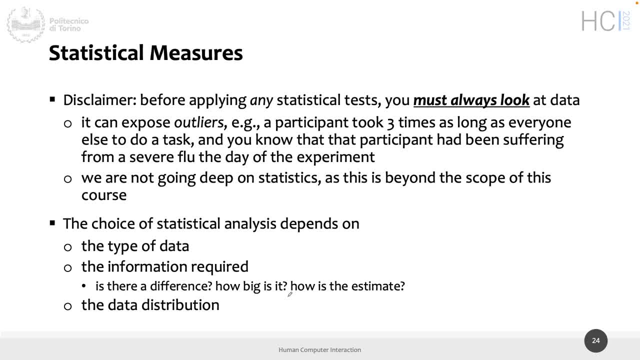 Or you had the computer continuously crashing for these participants. So it's the only one that is three times. So it's the only one that is three times slower than everybody else. So you can consider, for instance, to remove these participants from the analysis. 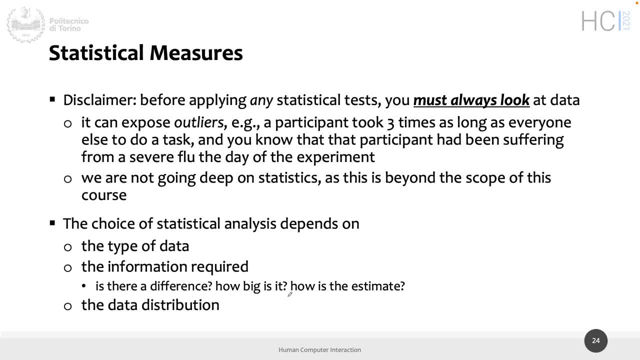 Because, for your knowledge, it could clearly be something out of scope. There are a lot of reasons- Computer crashing, the participants as distracted as issues, et cetera- that will produce this. So look at data And look for, let's say, for instance, outlier. 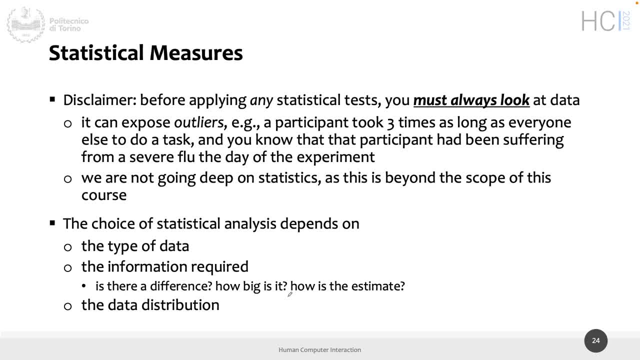 And then, once you have data cleaned, let's say you have to choose a statistical test. That depends on three things. The choice of statistical test- mainly The first one- is the type of data that you have. You have categorical data. 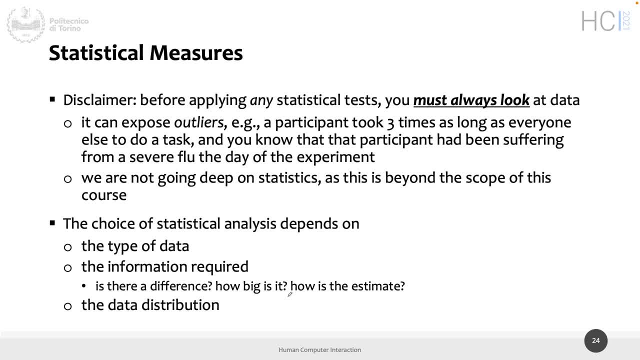 You have numerical continuous data or not. Some statistical tests work for some kind of data, others for others. Then the information that you require: Do you want to know if there is a difference, Or do you want to know, if there is a difference, how big this difference is, et cetera. 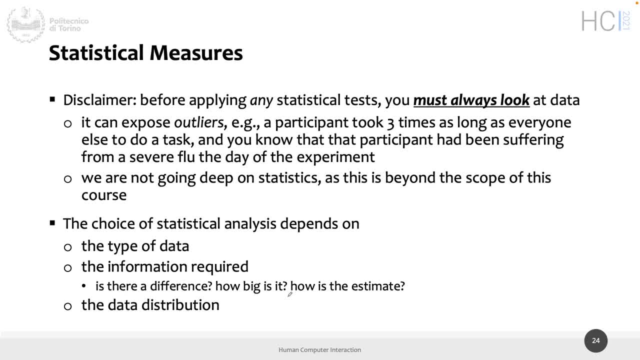 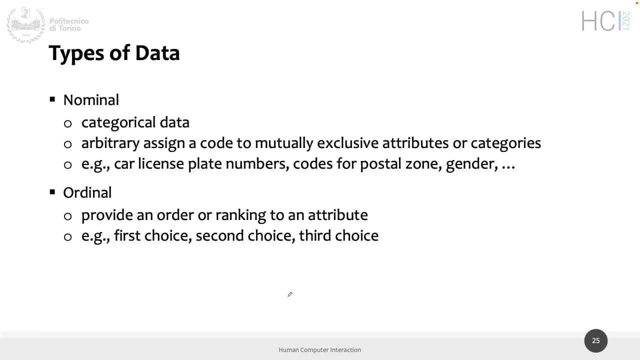 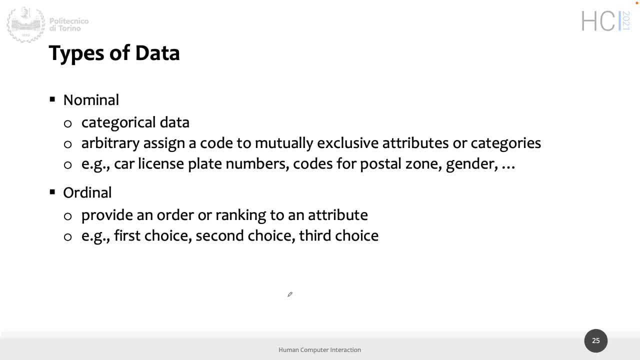 are arbitrarily assigned. You cannot say one postal code is bigger than the other. It doesn't make sense to say that the postal code of Turin, where Politecnico is, is bigger than the postal code of Via Roma. It is as a number, but it doesn't make sense to make this comparison. 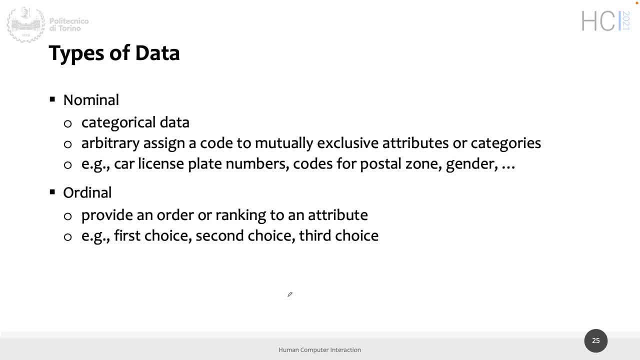 And this is the simplest way, the simplest type of data that you can have. Then you can have ordinal data, So data that is still categorical but provides an order or a ranking: The first choice, the second choice, the number one, the number two. 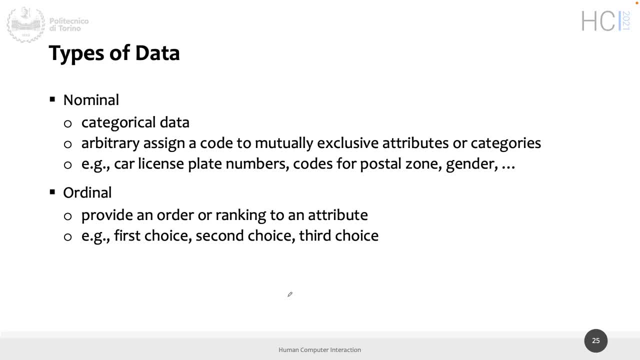 A, B, C, D in a certain setting. So at least you have an order. You still cannot say: maybe the first one is bigger than the second As a number. they are not, But the first one is more important. 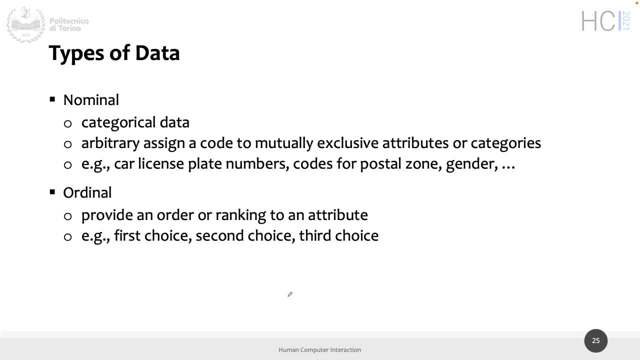 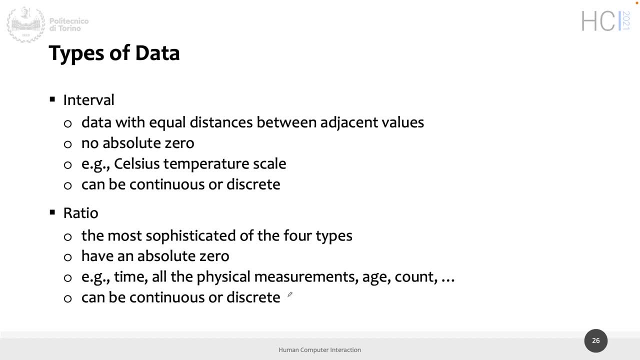 More popular, More something than the second one. Then you have interval data. You can build up in complexity. Interval data can be either continuous or discrete. So here you introduce continuous data And are data with equal distances between adjutant values. 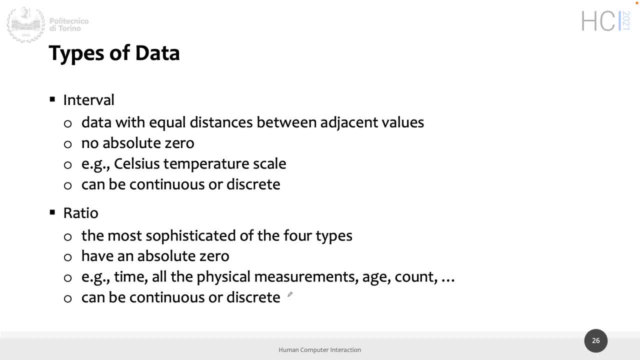 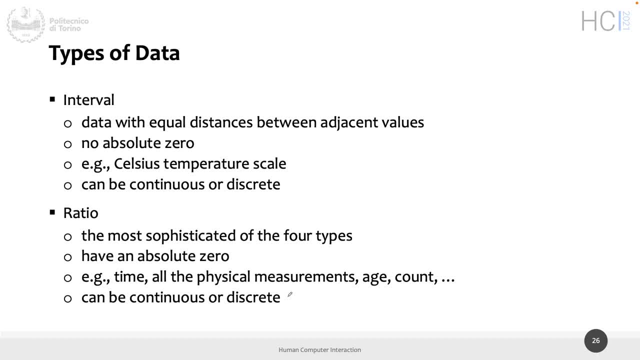 Because you go minus, Minus one, Minus three. You can continue with the scale. We know that in physics we will reach a limit, But the scale can continue In both sense. So this is an example of continuous interval data. 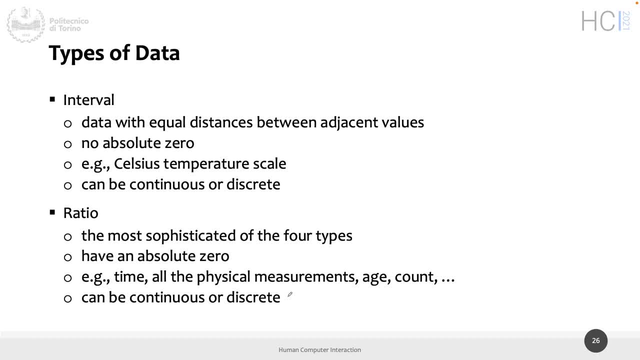 And then there is the ratio data. That is the most sophisticated of four And still has equal distances between objects and values And have an absolute zero. So time has an absolute zero, Age has an absolute zero. You can't say minus three years old. 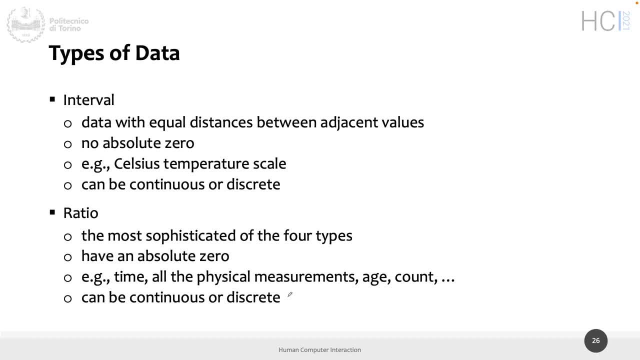 You stop at zero And all the physical measurements are typically ratio data And you can do different things. I don't know if it's in the Britain, Probably not. You can do different things. You cannot compute an average of nominal or ordinal data. 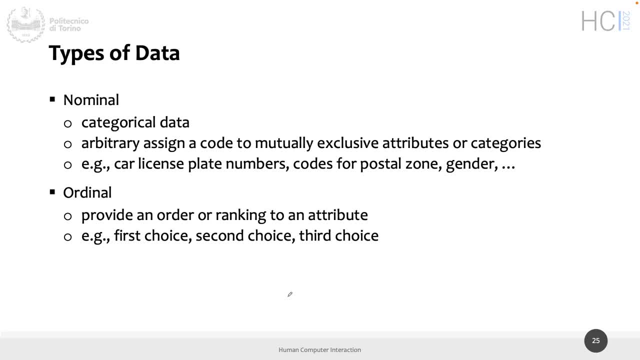 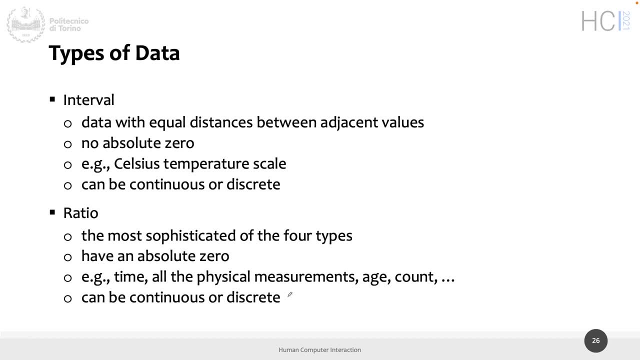 It doesn't make sense to make an average between two postal codes. You can compute the average Celsius temperature in a month. You can. It's reasonable to do that. You can compute the average of age of the people, Which is the average age of the people in this room. 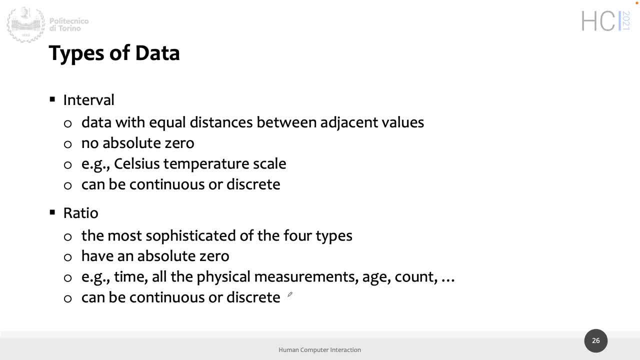 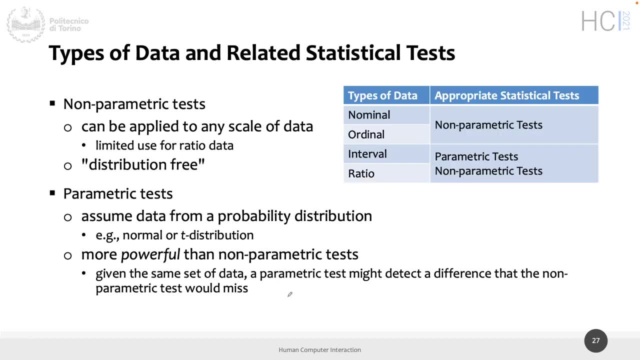 You can compute that. It makes sense. So you can do mathematically different things according to the different type of data. And according to the type of data you can apply statistics to kinds, to families of tests, And you can do nothing but this. 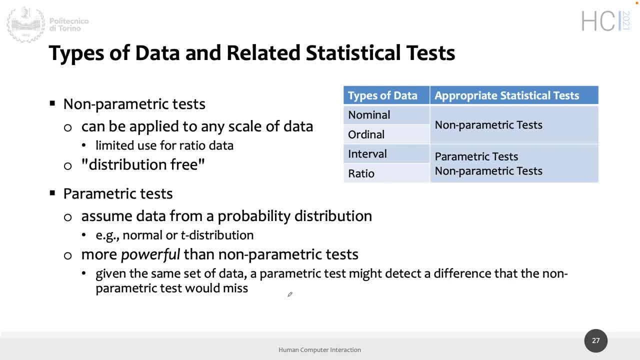 The first one is our non-parametric test that works with the simplest type of data: Nominal, ordinal data. You can only apply non-parametrical tests For the other two, the most sophisticated interval and ratio data- you can apply both. 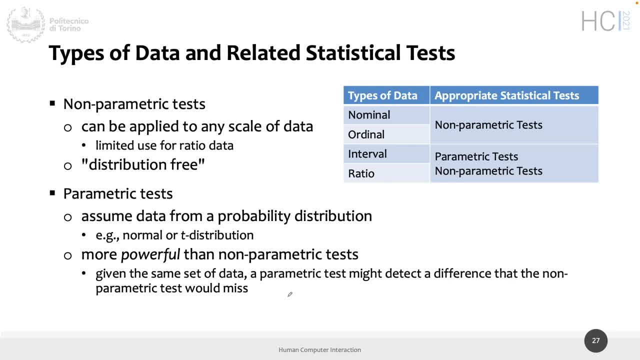 Either parametrics and non-parametric tests. So you can apply if you want nonparametric text for all kinds of data, but for parametric test you need at least interval, the interval category, the interval data. So nonparametric test could be used everywhere. but for ratio data, so if you collect information, 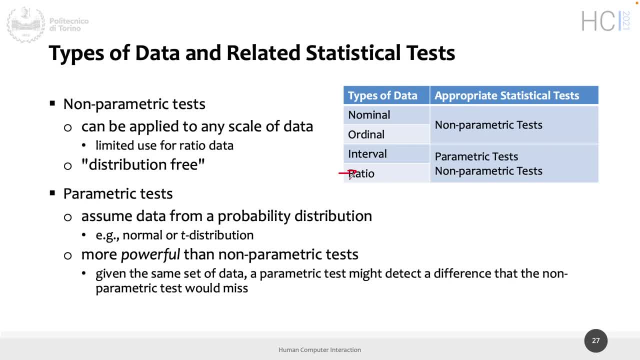 these are the information from your dependent variable, the things that you are counting for this kind of data, nonparametric test has a limited use. tell you very, very little about this data because nonparametric test has no strong assumption of the kind of data. 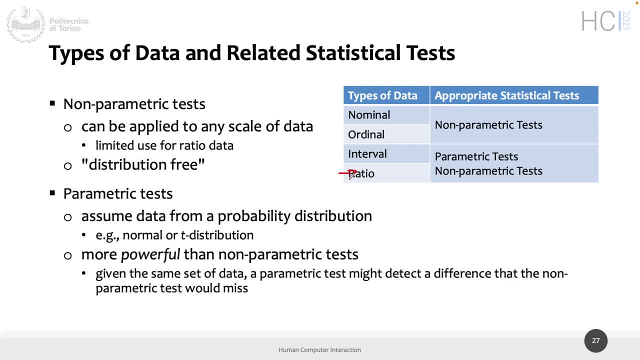 since you can use it also with postal codes, let's say, and can give you some information. Parametric test will give you much richer information, And parametric tests as a family are very useful. Both are surely more powerful than nonparametric test. 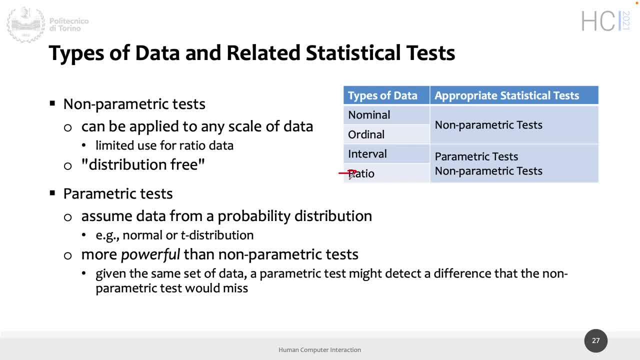 So, given the same set of data- interval data, let's say- a parametric test might detect a difference that is equivalent because there is an equivalence in methodology in the two families. an equivalent nonparametric test would miss. So if you have interval data and you have the opportunity to use a parametric test, 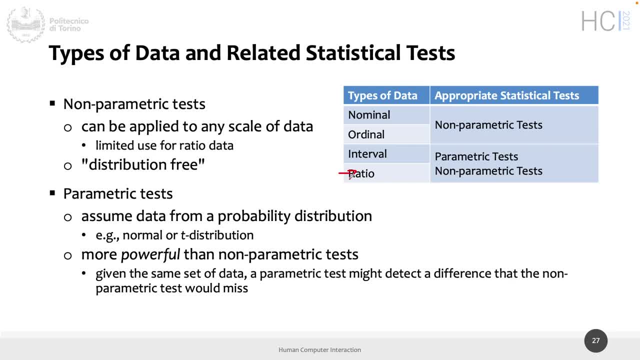 go for it, because the parametric test will give you more results, more insightful results than a nonparametric test. If you can choose, If you have nonparametric data or ordinal data, well, you cannot really choose. You can just use one kind of data, one kind of test. 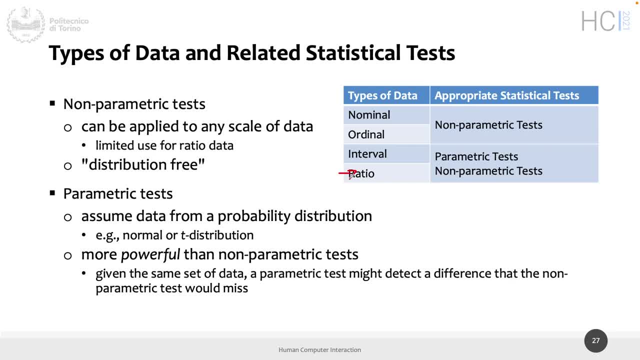 But they have parametric test. They are more powerful but they have assumptions And typically assumption that they have. then each parametric test could have a slightly different assumption than the others, but the main assumption is that data is under a certain distribution. Let's say data, the data that you collect is on a 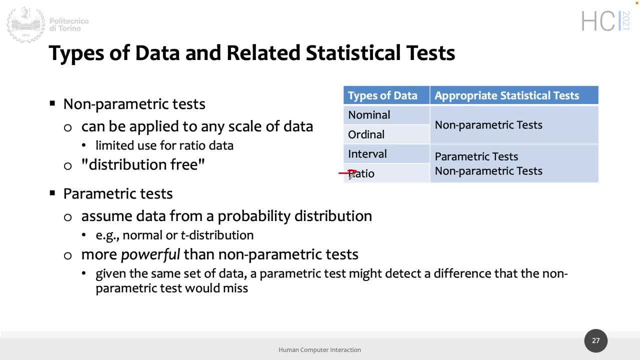 normal distribution, a Gaussian distribution, a t-distribution. They assume that there are some rules in data that are respected to be applied. So if you don't have data in that distribution, they don't really work. Some of them don't work at all, gives basically random results. Others are more. 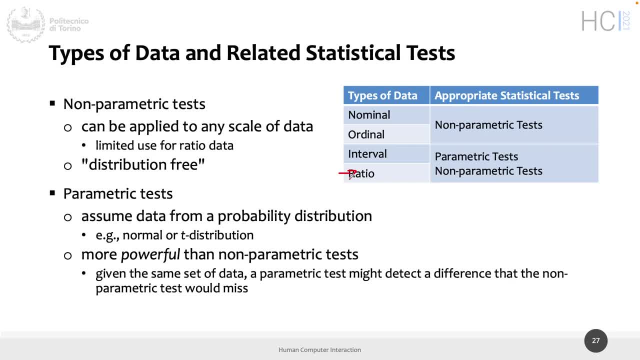 robust to change in the distribution. so maybe they work well with a normal distribution, but they still work well with a quasi normal distribution. so they're more resistant in that, But still they are more powerful. but they have some requirement. the non-parametric test doesn't. 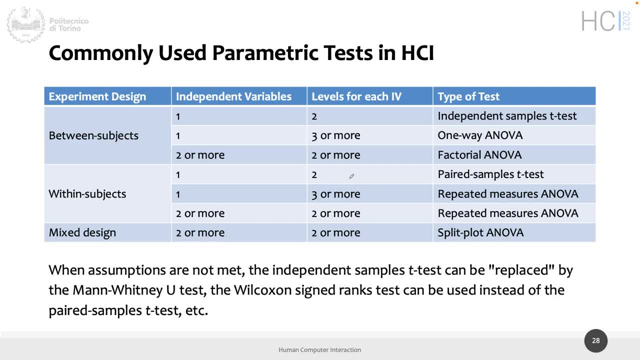 have. So, in a nutshell, which test can we use in our case where we have an experiment design, when we have independent variables that can change, etc. So this is a table of commonly used parametric tests in HCI that we are not going to see at all, that say: according to your experimental 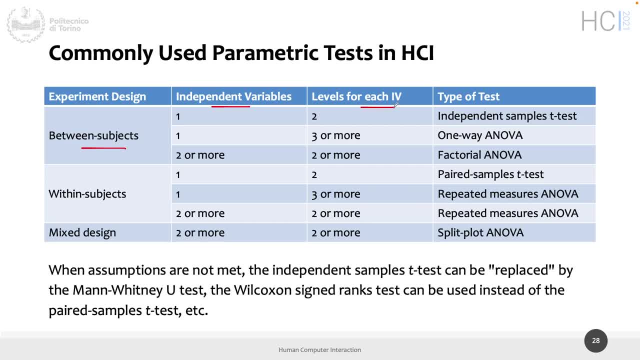 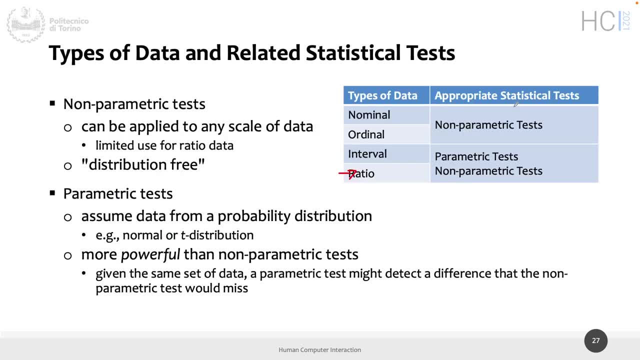 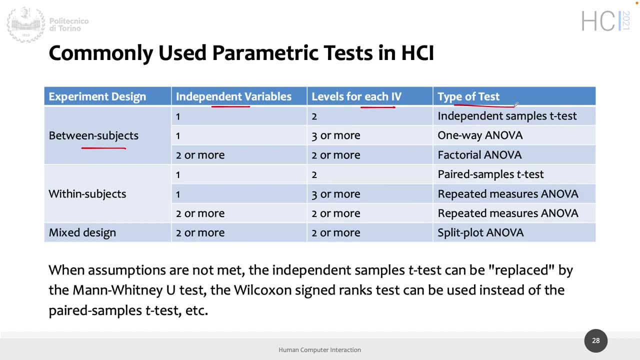 design variable that you have and the levels of each independent variable, assuming that you have either interval or ratio data- clearly not nominal or ordinal, because you cannot use parametric tests- and that your data has the right distribution, as this test asks you, or you can, in a way, modify or adapt your data so that they 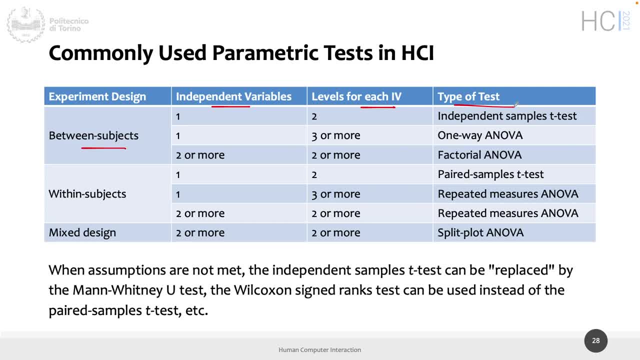 follow a distribution. you can use this test, for instance, in a between subject. if you have just one dependent variable with just two levels, you can use a t test. that it's even implemented in Excel, so doesn't really need anything fancy to be computed if you have still one dependent variable but you have a three. 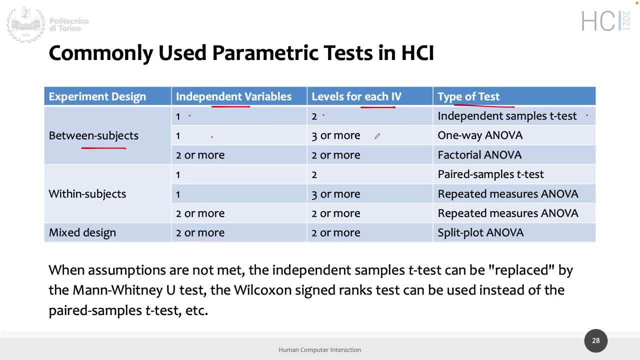 or more levels. you should use an ANOVA test, a one-way ANOVA test, not a t test, just one. one more level and things change. if you have a within subject, the things are repeated. if you have a within subject, you will have one independent variable, two levels. 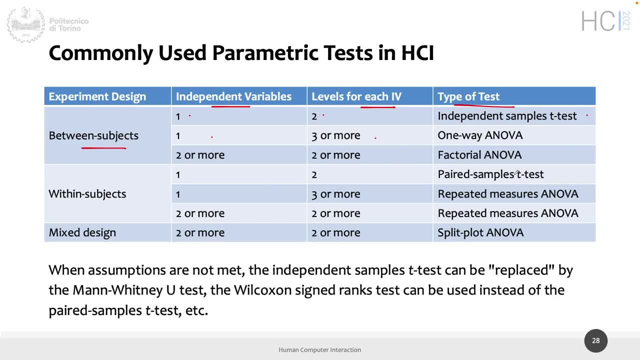 paired t test instead of a t test, the normal t test, and for the other condition, an ANOVA test, is slightly different because you have an within subject and if you have a mixed design, that means that you have at least two independent variable and at least two levels, because you cannot have a mixed design if you don't have at least 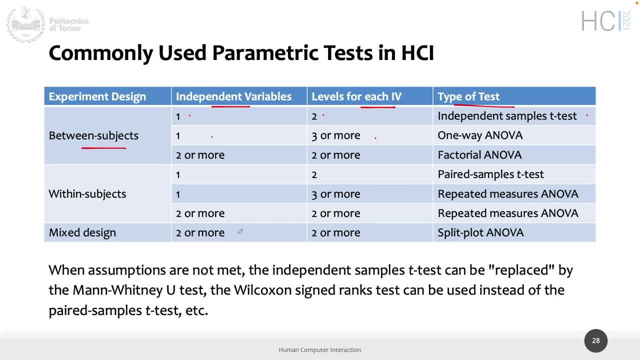 two independent variable. you typically use a split plot, ANOVA. so yet another kind of this ANOVA test, and these are the parametric tests, and each of them in practice, but also in theory, have an equivalent that is nonparametric, that can be used considering. 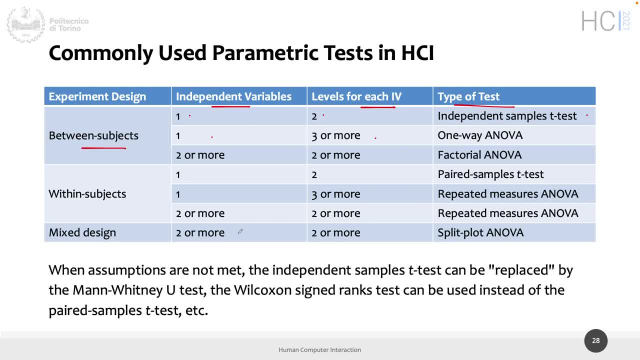 that it less powerful than the parametric test. so, for instance, instead of the paired sample t test here that is parametric, you can use this one, the Wilcox signed ranked test. that is another test that I have not assigned to you yet, but you can use this one. 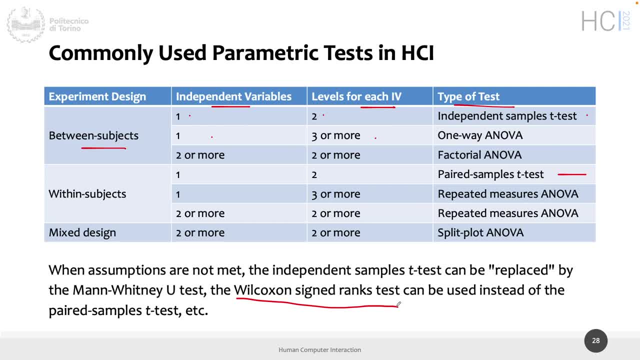 that is another test that I have not assigned to you yet, but you can do it on your own if assumption in the distribution of the data that you have collected And that you can use replacing to that. And all of these are standard tests, Tests that exist since years. 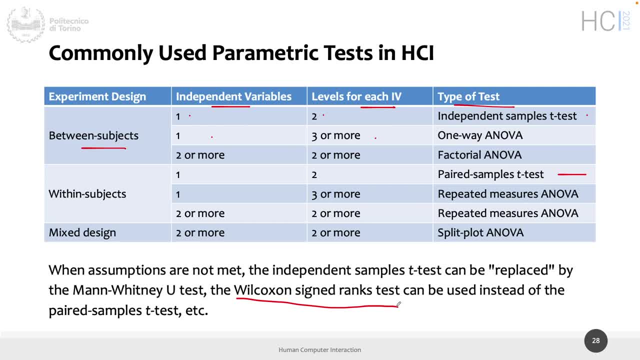 and years and years. Many of these are implemented, let's say, in Excel. You don't even need specific software to compute that. So t-test- the one way- ANOVA- is in Excel, for instance. The other kind of test- probably not. You need something more sophisticated than Excel. But for that 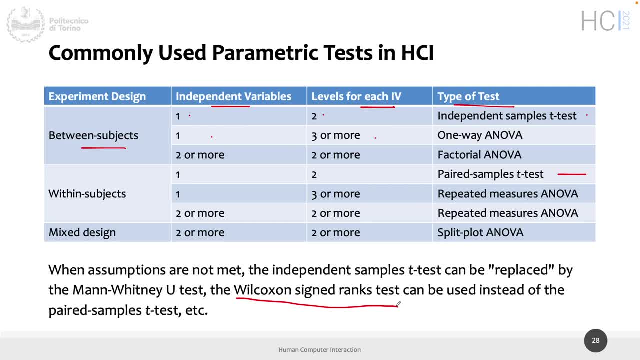 kind of things. just even Excel is enough. So this is just a table for a summary, Just in case you need to do a control experiment at a certain point. you have data. you have to analyze data as a guide to what to do. We, as I said, we didn't go, we won't go deep. 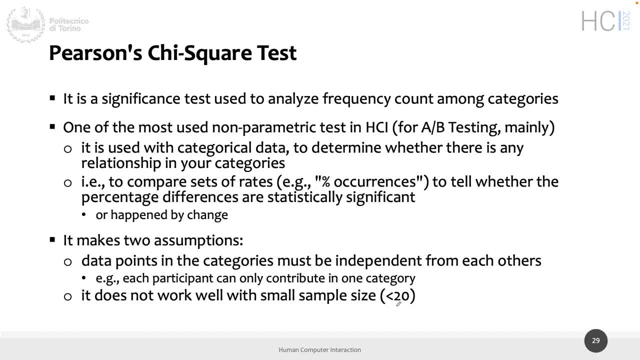 in any of this. We are going to see and we are going to do an exercise after the holidays on this test. That is a nonparametric test, So no assumption on the data Works with any kind of data And it's a test. But just to make an example of a specific test, Also considering what 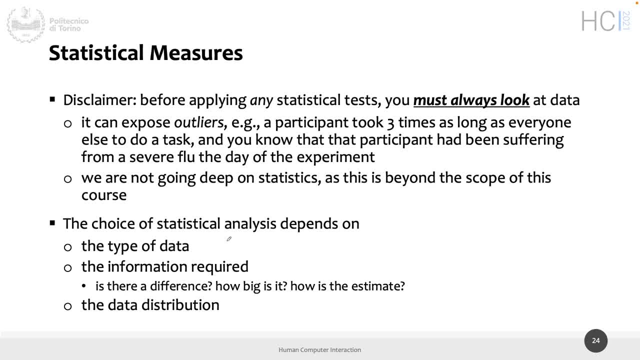 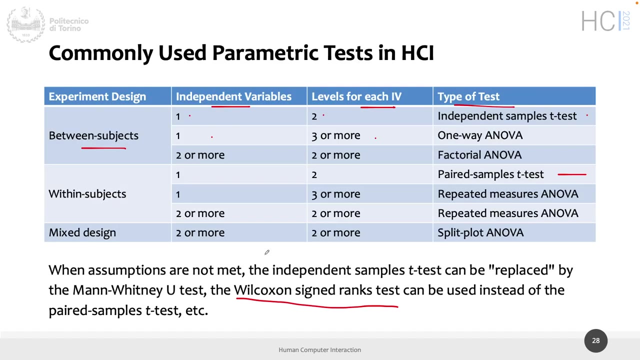 I said here That the choice depends on the type of data And we say that nonparametric tests apply to everything. The data distribution nonparametric test doesn't have really preferences for that, But this one, The information required, What this test can tell us. So this is a nonparametric. 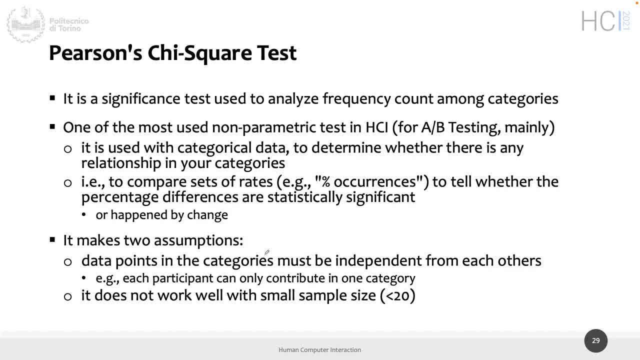 test. So it's not powerful a lot, But it's still one of the most used nonparametric tests in human-computer interaction And it's typically used for A-B testing. That could be the simplest way to do a control experiment. You have two versions of interface, Just two: A-B- Version A and version B. You 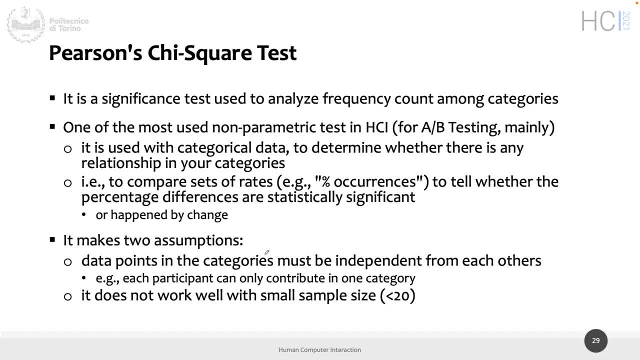 have two versions of interface. You have two versions of a button. You have two versions of a menu. You just have two versions. That is still a control experiment, because you have just one independent variable with two levels. So it's simple, But you have two versions. 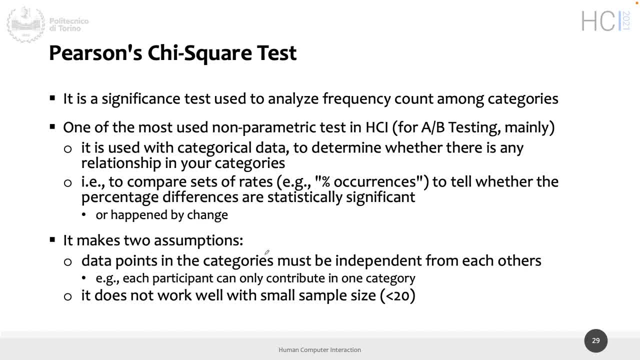 Hmm, And one of the most use for doing this kind of thing: A versus B, Which is better in a way, And it used with categorical data To determine whether there is a relationship in those categories. Doesn't say which category is better. Doesn't say if A ‑‑ if A is. 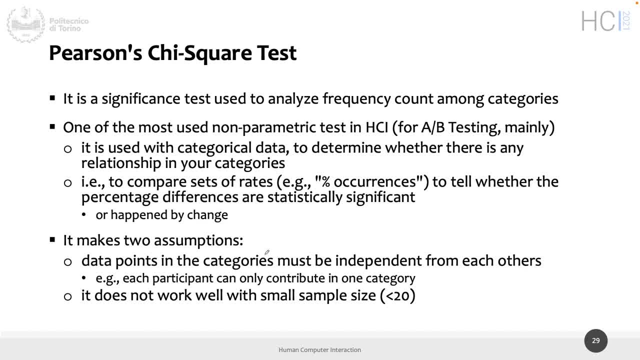 three times better than B. It just says there is a difference between A and B And probably A is better. But that is How much better according to the data you collect? This test doesn't tell you, Just tell you that there is a difference. So 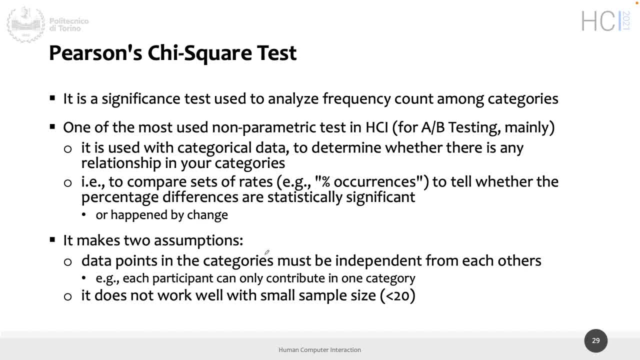 you can, if you have a null hypothesis, reject a null hypothesis and accept the alternate hypothesis, And this is to determine whether there is a relationship. more formally, is this one The chi-square test? compare set of rates. So the percentage of occurrences in your measurement in case A and in case B to 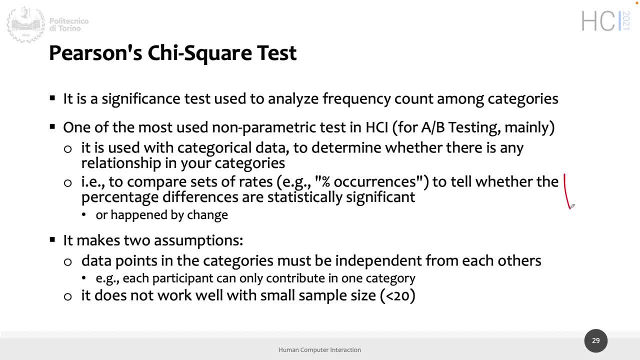 tell you whether difference between these two percentage are statistically significant or happened by chance. You have eight people in clicked on the button in interface one and four clicked in interface two. So 60% versus 40%, let's say, Or 70% versus 30%. 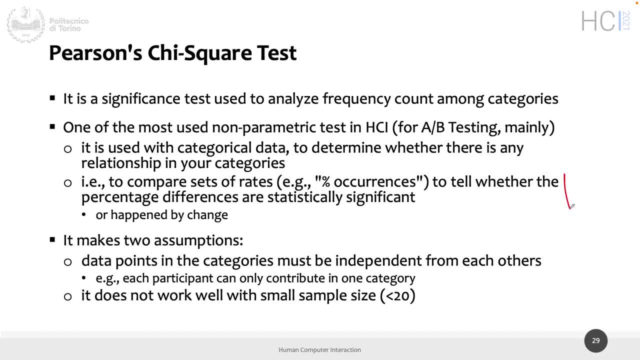 Is this number random or they are really different? If we do the same experiment, as I said before, with another group of people with the same characteristics, with the same interface, I will get a result that is more accurate. I will get a similar number, So a preference for the first one versus the. 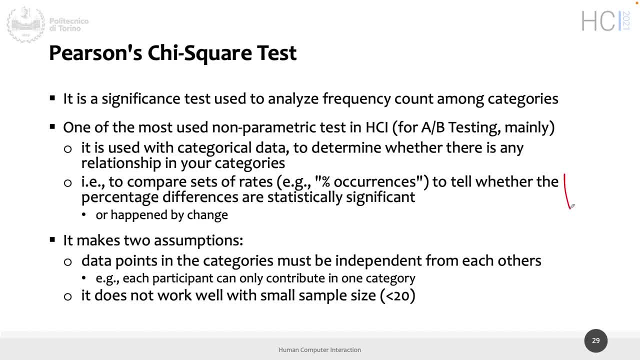 second one, or not? Chi-square say, allow us to answer this. To answer: yes, there is a difference, But not again how big this difference is, But there is. So A is better for what you measure clearly than B, And it makes two assumptions It. 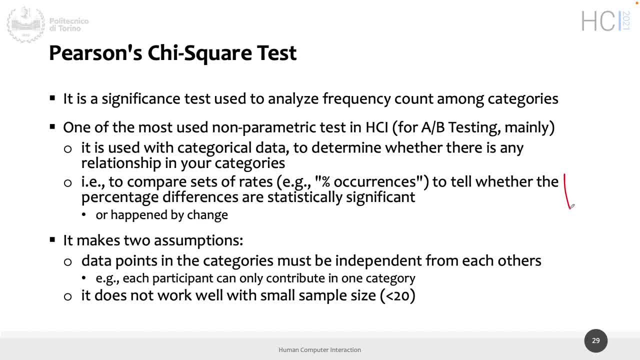 really makes two assumptions. So still, even if it's not a parameter test, it makes two assumptions that must be met. The first one is that it doesn't work well with small sample size, So you need to have more than 20 data point. If you have less. 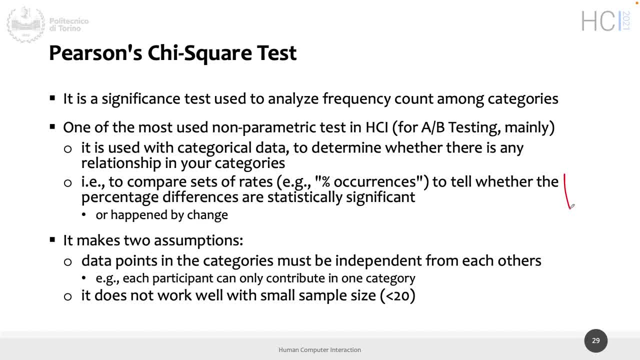 than 20, it works. It can do the math, but the results are not really useful. They are not really precise. let's say You need to have at least 20 points. 20 measures And data points in the category must be independent from each other. 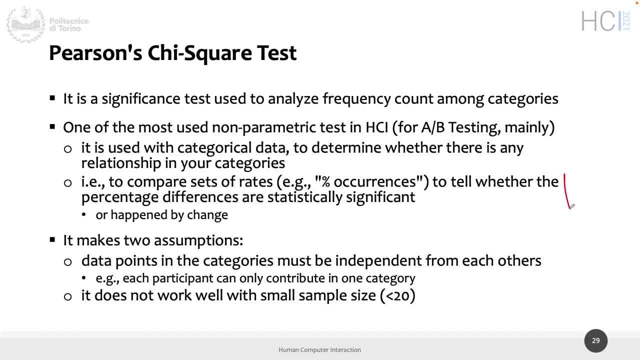 That means that each participant can only contribute to one category. So if you have version A and version B, one participant can contribute to one category. If you have one participant, one participant can contribute to one category. If you have a second one. 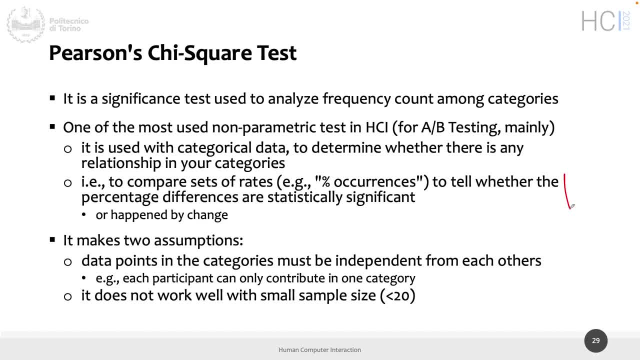 participants cannot do A and B in the same moment, Can either see A or B. These are the only two assumptions that this test is doing. So let's imagine to have the portale di didattica, the same portale that you have just with I don't know, instead of the title material. 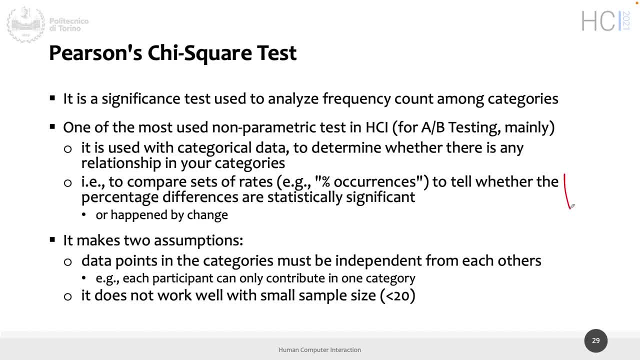 in a course description. you have also another title, So half of you will see the label material and the other half of you will see something else instead of that label, And Polytechnico could be interested if it creates more engagement material or the other label. So if half of 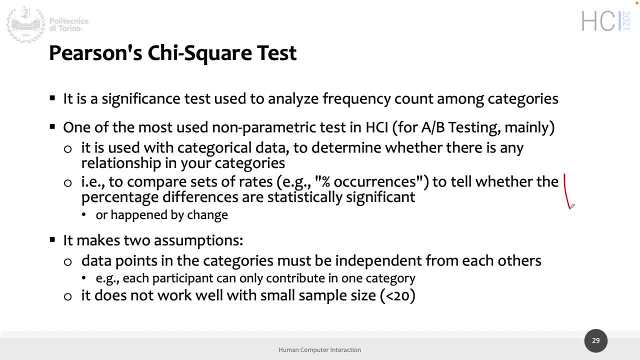 you click on material more than the other half of you. CanSquare test can tell us if this difference is the same, If there is a preference between one and the other version in terms of this kind of engagement that we can measure, for instance, with number of clicks. But you can do this. 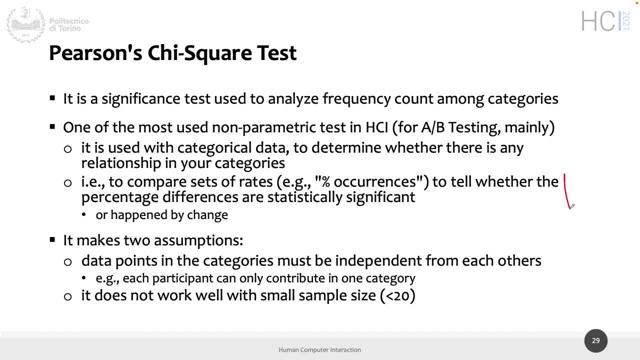 because you are a course of 100 people. So we have 50 and 50. That is way bigger than 20.. If we just do this here with the person people present here, you cannot do this because you are less than 20.. So these are just the two main assumptions. 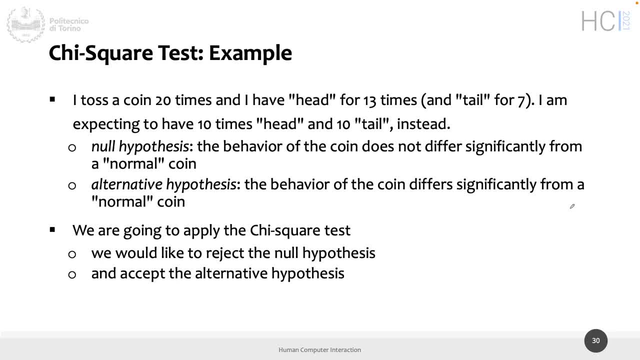 So let's make an example of how to use and apply this chi-square test. Moving from user interface to money. I toss a coin 20 times. I take one euro and I toss the coin of one euro 20 times. I do an experiment: Take one euro and I toss the coin of one euro 20 times. 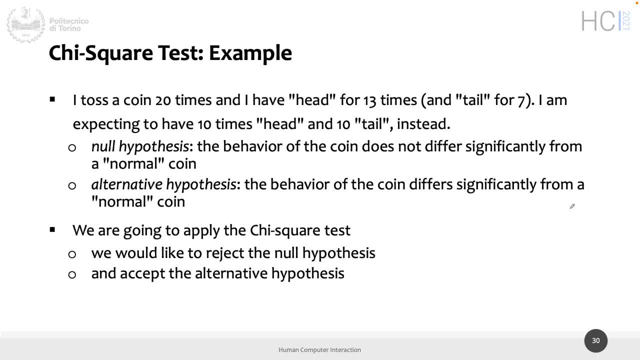 I take one euro and I toss the coin of one euro 20 times. I do an experiment: Take one money, Toss the coin, launch the coin and 20 times And for 13 times I have head and for seven times clearly the other I will get tail. I toss it 20 times. 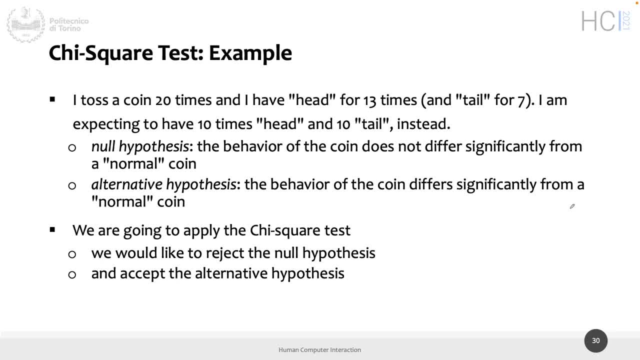 And this is my experiment And I also have, let's say, a ground truth, Right, If I toss a coin, I toss. what do you expect? It's written here, but what do you expect? How many times should came head or tail. 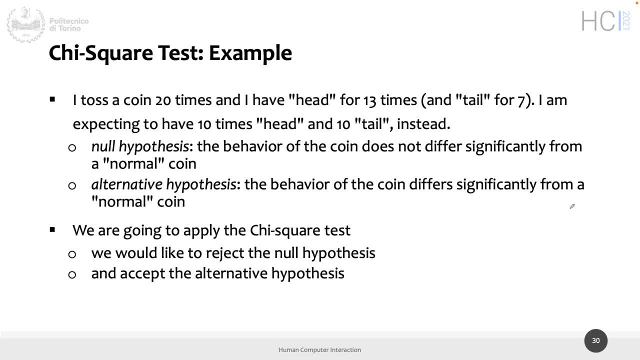 10. If you toss a coin, you're expecting that 50% of the time you get head and 50% you have tail. Instead, in my case, I have 13 versus 7. It is not 10 and 10.. So my 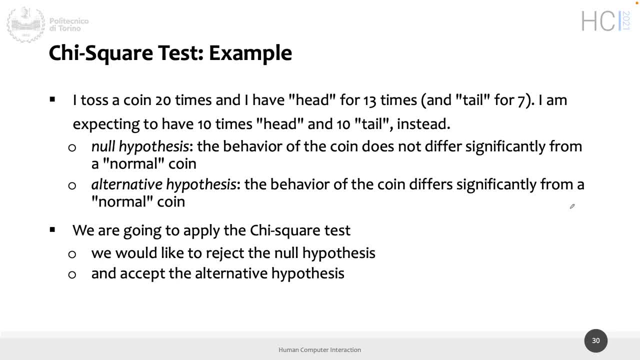 hypothesis is that the behavior of my coin. my hypothesis is that my coin is fake. It's unbalanced as a coin, it's not a normal coin. So my alternative hypothesis is that the behavior of my coin differs significantly from the behavior of my coin. So my alternative hypothesis is that the behavior of my coin differs significantly from. 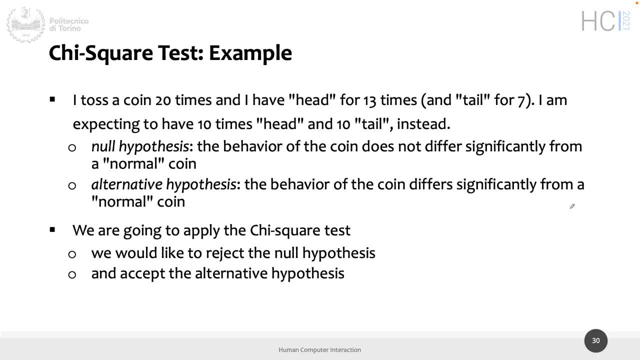 a normal coin Dependent variable: the number of launches of tossing the coin, The null hypothesis. you see here an example. the behavior of my coin does not differ. It's the same as normal coin. So this number just happened by chance And 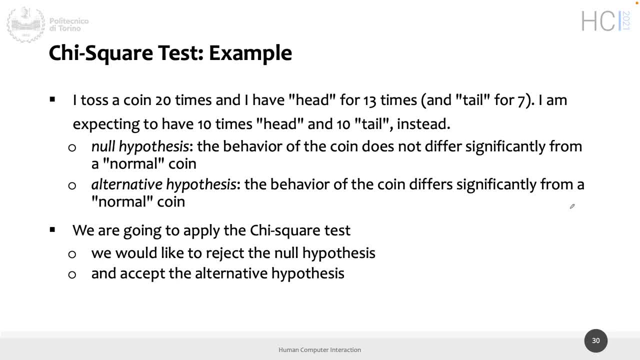 we are going to apply the K-square test and we would like to reject the null hypothesis and clearly our goal is that: to reject the null hypothesis so that we can demonstrate that my coin is fake, it's unbalanced, it's unfair as a coin, it's not a normal. 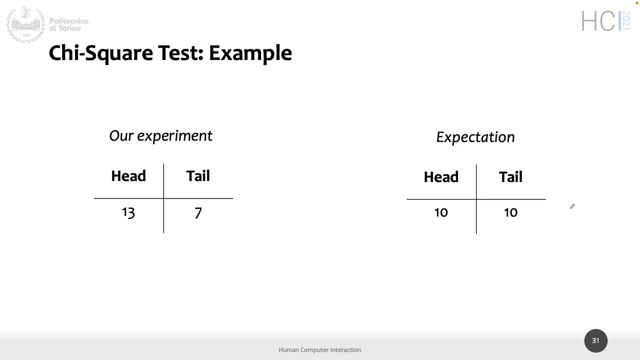 coin. So this is what we can write. We can write the table head and tail with our experiment here, which say, okay, head 13 times tail 7, and clearly the sum is 20.. And we have also the table with the. 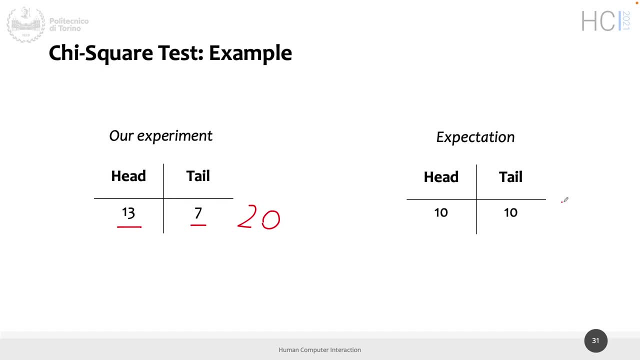 expectation, which should be clearly the sum must be still 20.. This is important. This is obvious here because we toss a coin 20 times, but in general, this is important. The experiment and the expectation, the ground truth, should be the same: 20 and 20.. 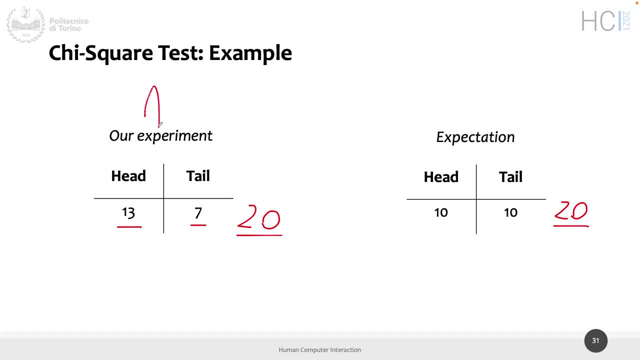 So, in a way, we are doing A-B testing: This is A and this is version B. in a way, Clearly, this is not an interface, But we have an experiment and we have an expectation. Okay, So we have numbers, we can. 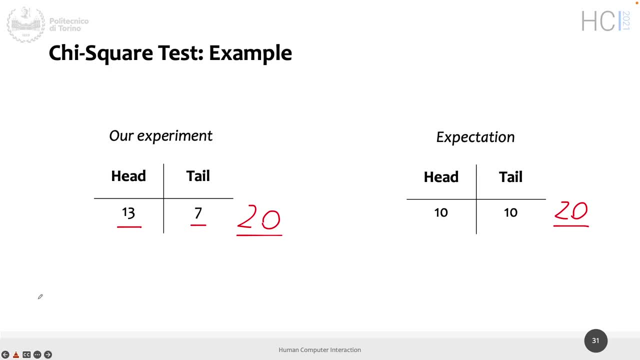 write this table. So if, instead of a coin, we have interface, we can measure time, And so here we will have time of version 1 and time of version 2.. So it's A-B testing here, not there. We have A and B, head and tail, Interface 1, interface 2. But we have our 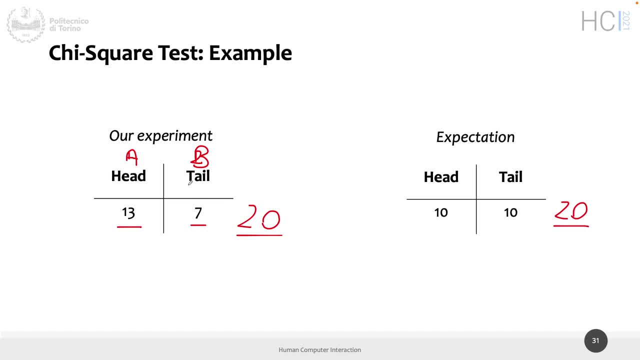 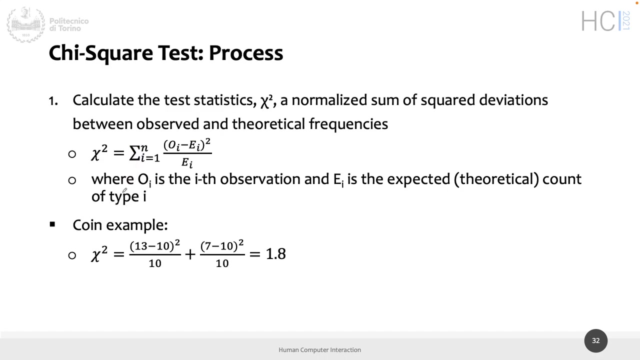 experiment and we have what we expected to be the failure expectation, in this case for coin. it's easy. So here we have numbers, but again in a user interface we can add speed, time, number of clicks, number of errors, etc. our dependent variable. So how we can proceed, How it works as a chi-square. 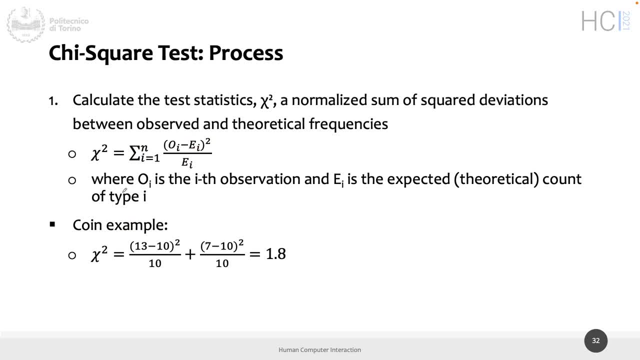 So, first of all, we have our 2013.. This is the processor that was installed for the, For example, chi-square is this formula here? It's a normalized sum. it's called chi-square because this symbol in Greek is called chi. 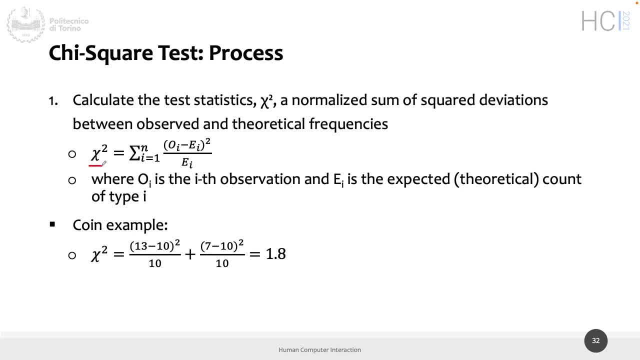 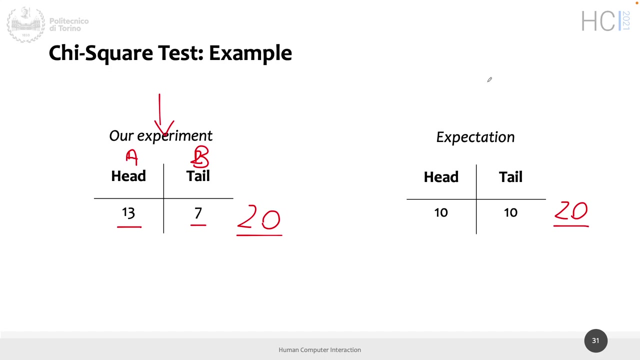 It's written as the Italian chi C-H-I. It's chi-square because chi power two. Chi-squared it's chi-square test. So this is a normalized sum of the squared deviation between the observed and the theoretical frequencies Between the observed. our experiment. 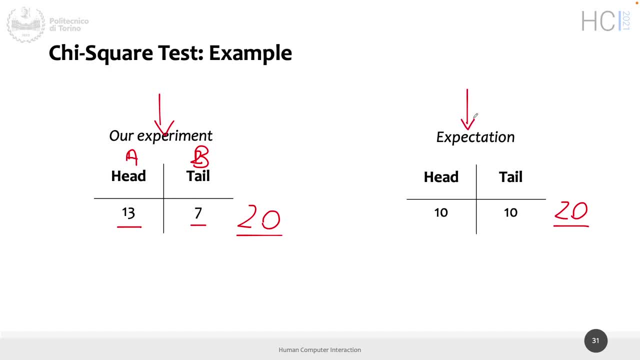 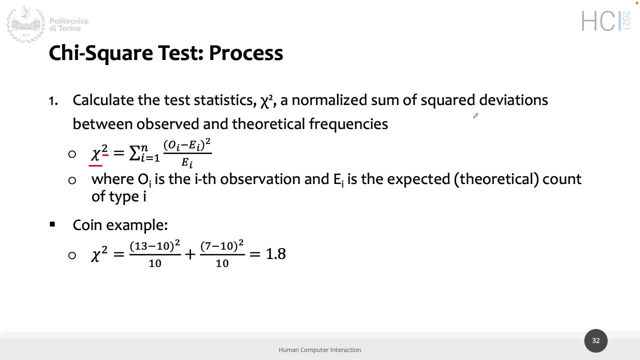 and the theoretical, the expectation. So what we get versus what we expect to have, And we need both because the chi-square formula ask us for both. So basically, in our coin example, this is what we are going to do. We just have two cases. 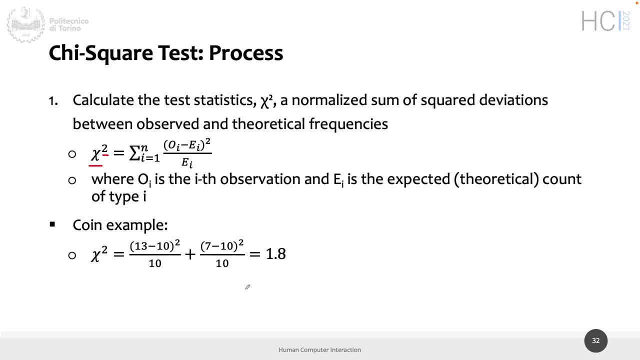 Head and tail, So it will be 13,. our number of head with our coin, minus 10, the expected number of head squared divided by the expected number of head, That is 10.. Plus the same things for tail. 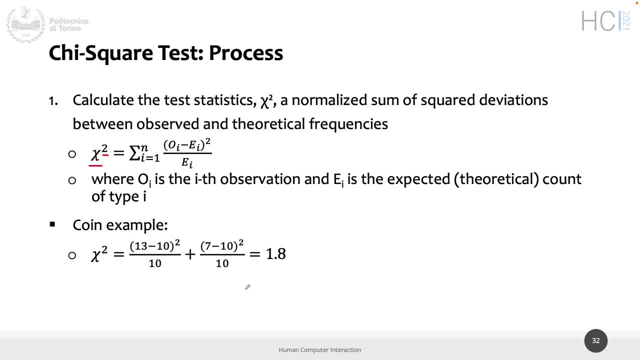 Seven our numbers minus 10, the expected value squared divided by 10.. In this case, the expected value for head and tail is 10.. If they will be different, we will have different number, clearly. So if you do all these computation, 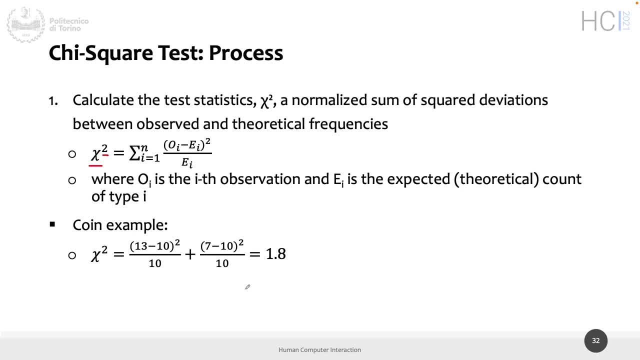 and you round a bit, you get 1.8.. That is a nice number, right, And it's also useless up to now. But you calculate that And this is the number, that is, the chi-square 1.8.. 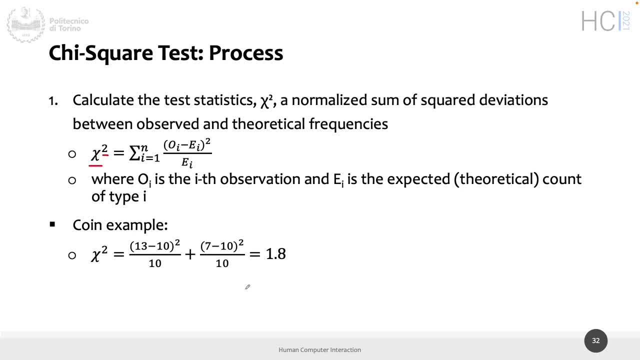 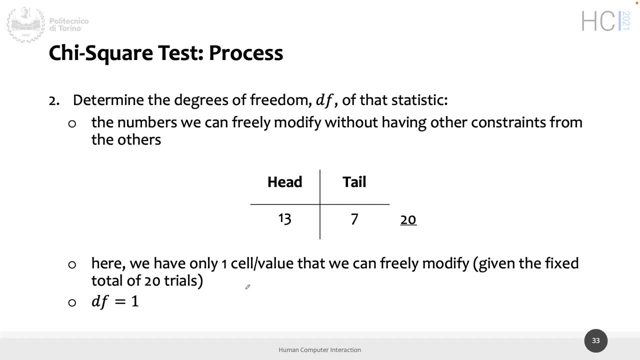 What you do with that. You need, before understanding what to do with that, you need to determine the degree of freedom of that statistics, of that observation. What you do is, you should do 5.8.. For example, 10.8.. 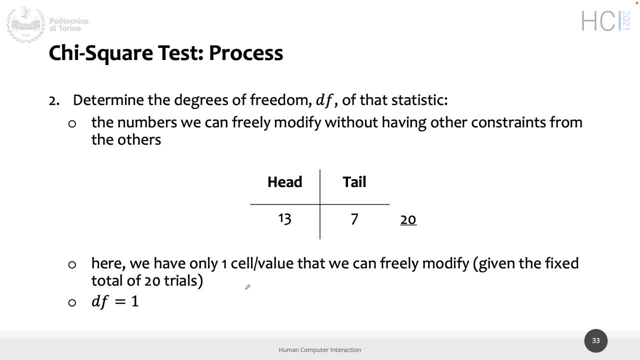 For example, 5.8.. that computation that you did and the degree of freedom is the number, the numbers of in this case is the number of numbers that we can freely modifying without having other constraint of the others. so here we have unconstrained, which is the constraint here. 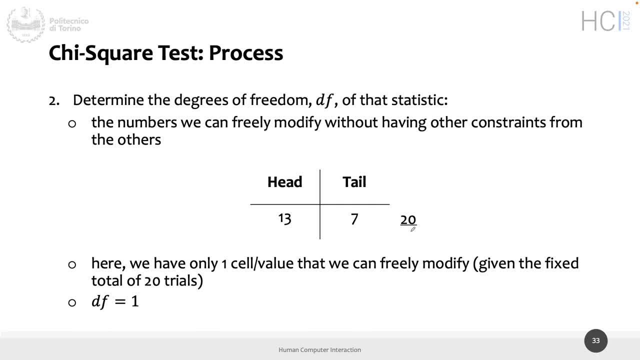 we have just one constraint in this table, which is the constraint yes, there, yes, the constraint is that the sum should be 20 because we toss the coin 20 time. so that is our constraint. we cannot have. so if we change head, tail should be the new number 20 minus the 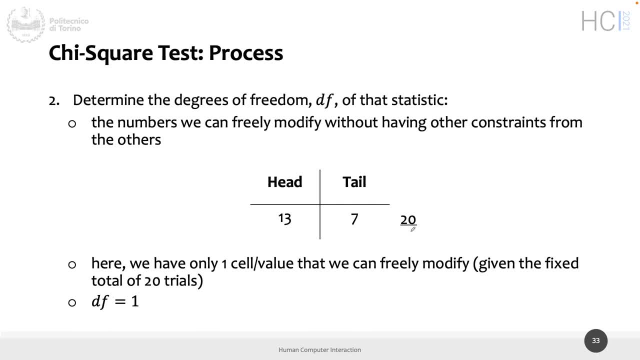 new number because the coin are just head and tail and so if we change- and we did it- 20 times, so we cannot have anything else. and if we change tail, same things. head is constrained by the number 20. so here, how many numbers between these two. 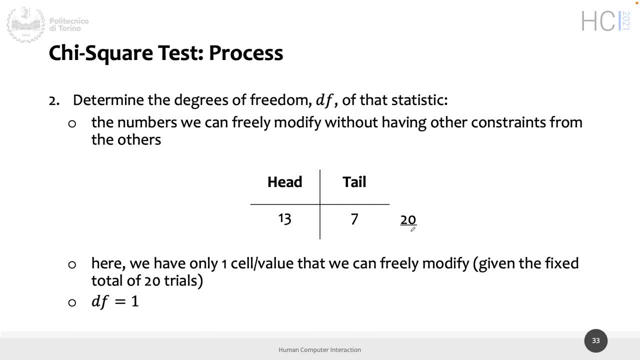 so here, how many numbers between these two we can freely move without having other constraints? for the numbers one or two, how many numbers in this table can we? so if we change here these hypothesis? not one, we have one, it's. it's Britain. so ok, it's one. so we have just. 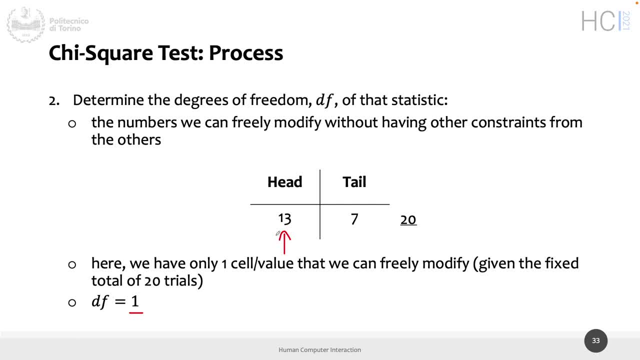 one degree of freedom because we can change just one number. it's one degree of freedom, is our number and we can move freely and we can move with it. we can move freely and we can move with it just one number freely: We can change 13,. but if we change 13,, 7 is not free to. 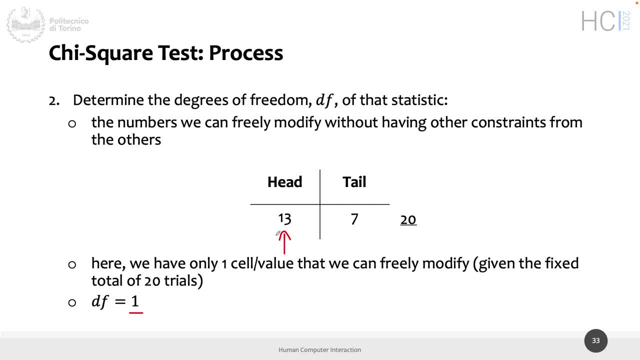 move because it's constrained by 20.. And if we change tail, head is not free to move because it's constrained by 20.. We cannot have 5 head and 3 tails because the sum must be 20, because we toss the coin 20 times. So in this case we 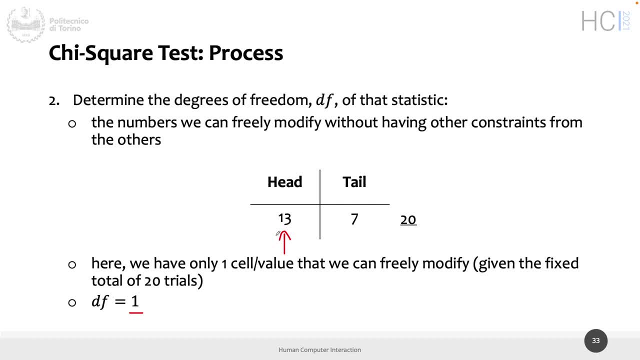 just have one degree of freedom because we can freely move one cell in this table. If we could move both in some case without constraint, so putting head 3 and tail 5, freely, then we would have two degree of freedoms. but here we. 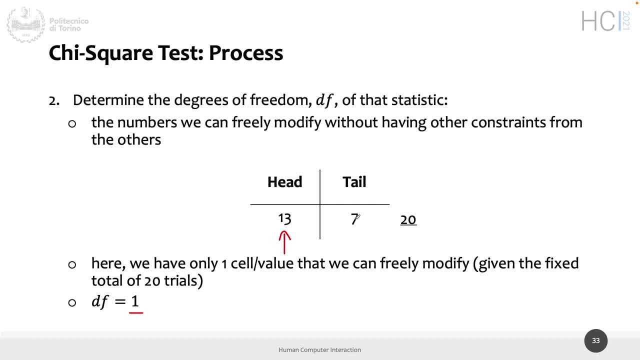 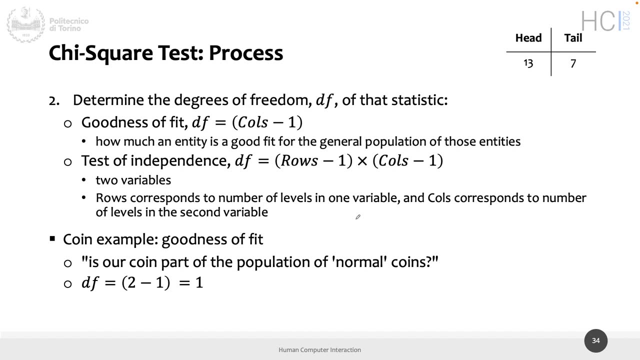 cannot. One is free and the other is not, And that is constrained by the number of tosses that we made. Is this clear? The degree of freedom? Yes, This is intuitively. mathematically, there is a formula to compute the degree of freedom. 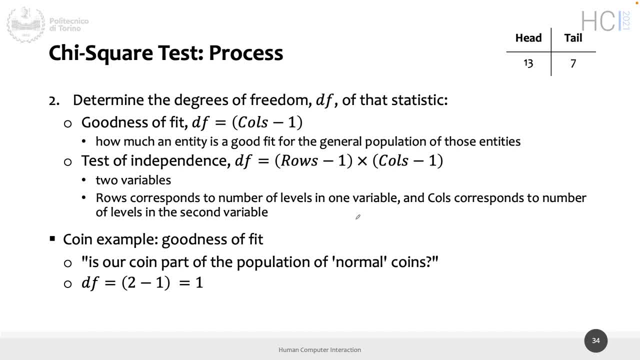 That is a way to check, especially in A-B testing of something like that, if you apply the formula properly. And we have actually two ways of computing the degree of freedom. The first one is called the goodness of fit and is number of columns minus one. 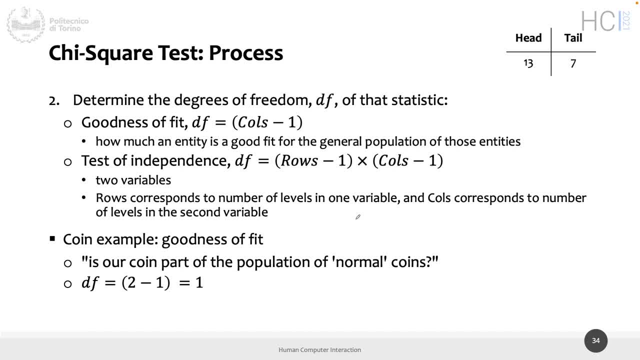 And the other one is the test of independence, That is, number of rows in this table. number of rows in this table minus one multiplied by number of columns in this table minus one. Basically, for the goodness of fit, can be used only when you have one variable. 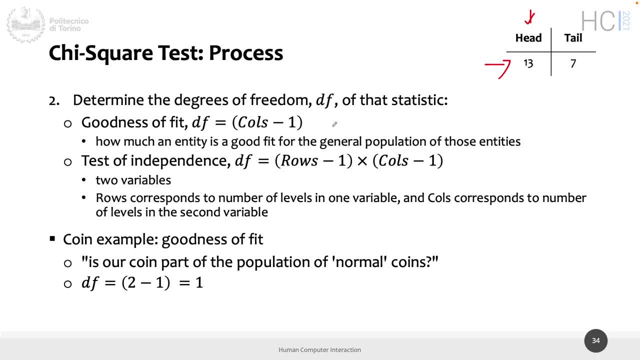 Like in our case, We just have one row, So the second formula will be zero plus multiplied by something else. So in this case we use the goodness of fit and our results is one. But actually in our case we use the goodness of fit. 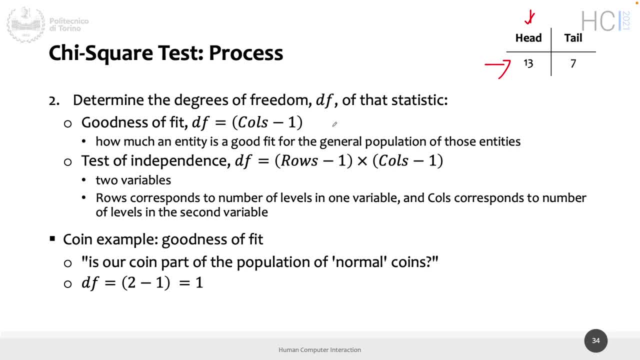 And in A-B testing we typically have the degree of freedom. that is one, Because we typically have A and B, So in any case we have. often we have one as degree of freedom. The difference here is that the meaning behind the goodness of fit and the test of independence 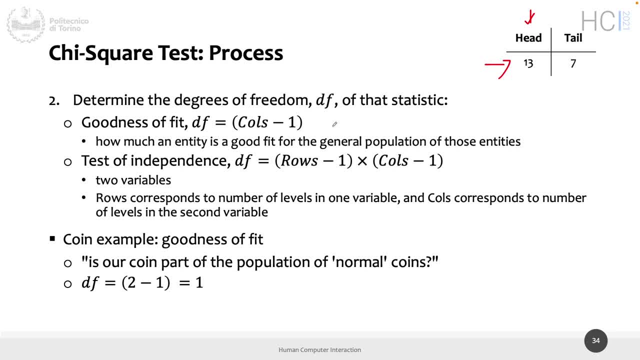 The goodness of fits, say how much an entity is a good fit for the general population. Basically say how much a coin is a good fit for the population of coins. That is actually our case. We want to have the goodness of fit Because we want to understand if my coin is part of the population of normal coins or 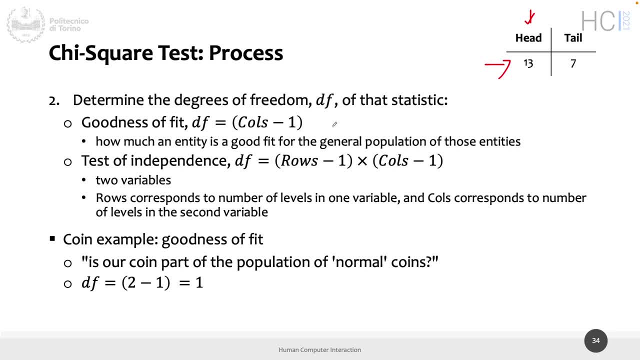 not. So we want to compute the goodness of fit. So we want to compute the goodness of fit. So we want to compute the goodness of fit. So in this case, the table and the formula are well aligned, because the goal is the one. 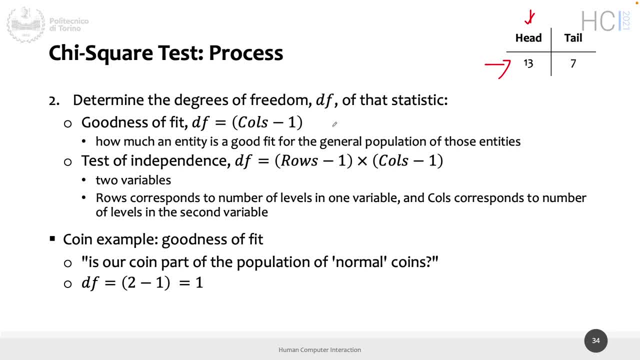 that used the formula. If you have two or more variables, you can still use the goodness of fit. You ignore the rows But you use the goodness of fit if you want to get this information, If you want to get if an entity is a good fit for the entire population of the normal. 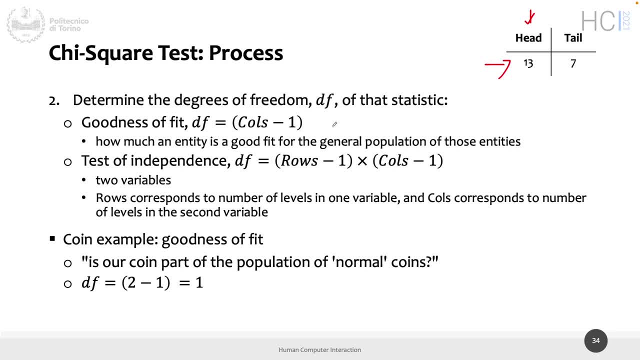 let's say entities Like in our case. Hmm, So in our case it's a goodness of fit. We want to know if the coin is part of the general population of coins, So we can say 2 minus 1, 1.. 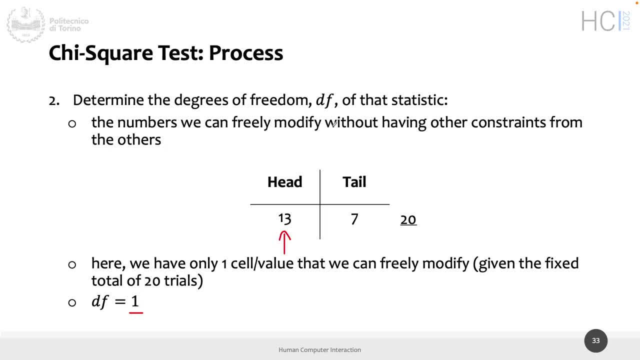 And again, if you want to prove, this is the way to prove that In both cases, Both in the test of independence and in goodness of fit case, This work, this intuitive calculation, work in both cases. But if the table is bigger you just have to pay more attention here. 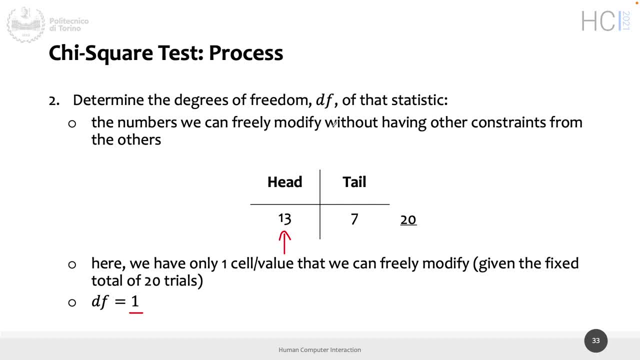 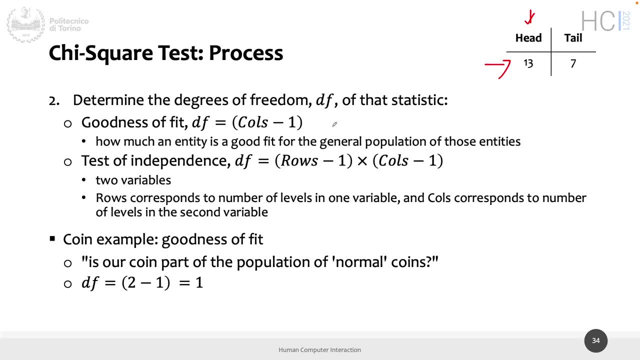 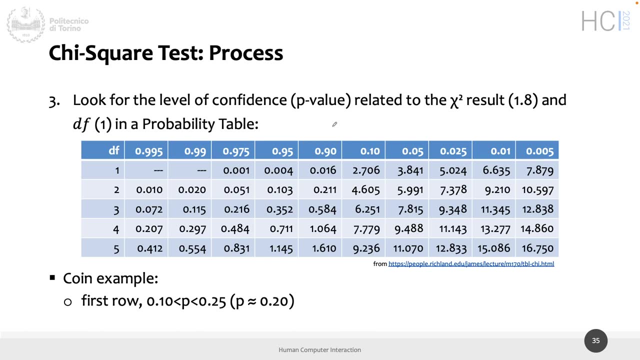 Hmm, Which one to count the number of numbers that can move freely? So in our case it's 1.. So we have two pieces of information now. We have our results of the chi-square, that is 1.8, and a degree of freedom that is 1.. 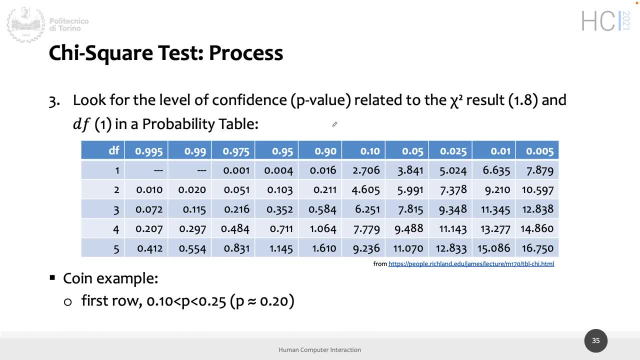 What do we do with these two pieces of information We get together with the chi-square test. we got a table like this, Bigger than this: Hmm, This table continues here after 5, and that's probably something here in the middle. 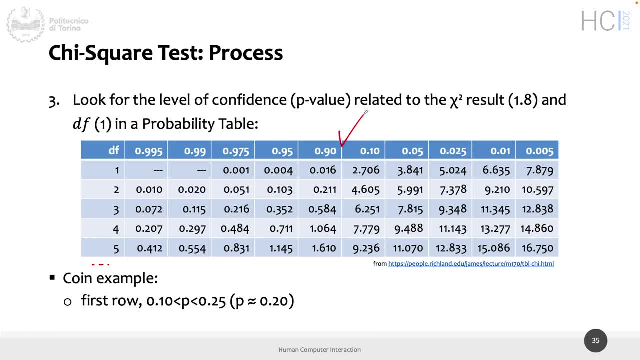 0.9,, then will be 0.8,, 7,, et cetera. It just cut here in the slides, But there is the reference here to the full table that is pages long. So what we want to do here is to look for those two numbers in this table. 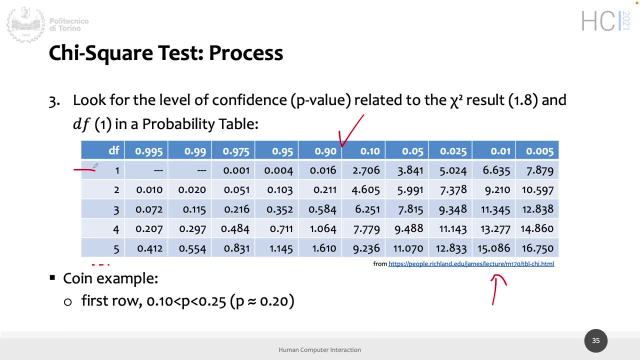 Hmm, So we have degree of freedom 1.. So we need to look at the first row. If we add degree of freedom 2, we need to look at the second row clearly And we should look where is the result. Hmm, 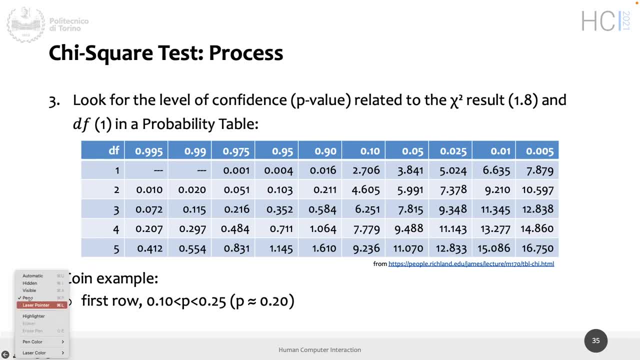 Let me delete this one second. So first row here And we need to look where is the result: 1.8.. Where is 1.8 in the number of this row? Right here In that row, It's not there. 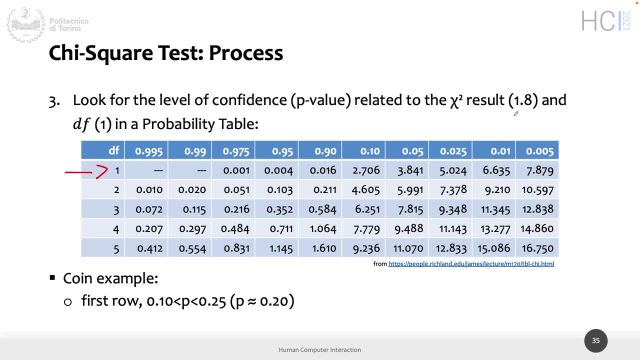 Right, But it should be something here in the middle, In the portion of the table that is missing. Hmm, So this is 2.7, this is 3.8,, this is 5. So there is more or less 1.5 in the middle. so it should be around here. 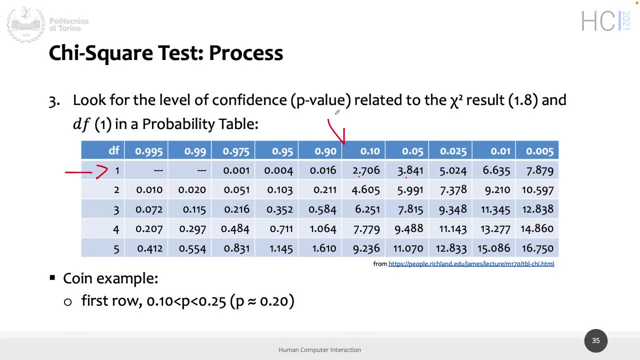 Hmm, 1.10 and 0.25 if you look in the table is. you still don't have, if you look in the table, the precise number, but the 0.25 should be something like 1.6, let's say. so you look in the table where there is, which is the interval that you have. 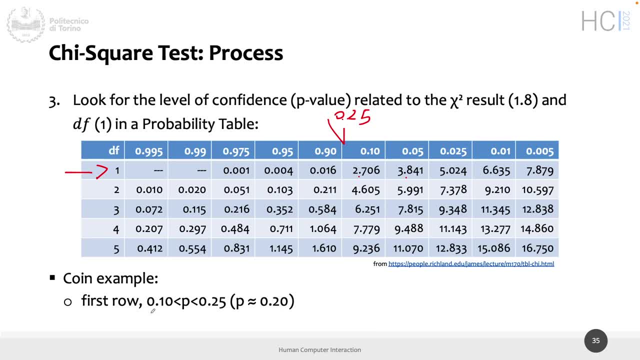 and you can say that your number 1.8, is, let's say, included between 0.10 and 0.25, and probably it should be something around 0.2. so if we here we had not 1.8 but we had 5, well it's surely there, but we have 1.8 in our. 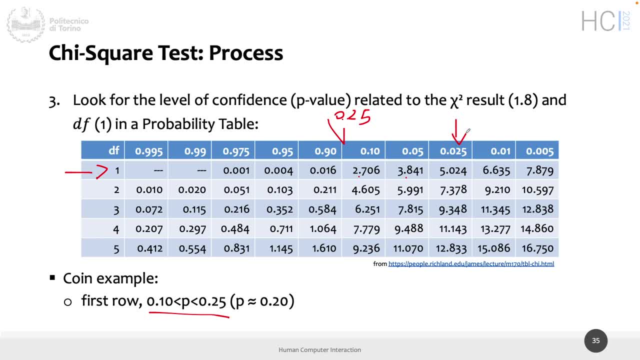 computation. so you're just picking this table where the number is in the right row. so, okay, we have yet another number we have. this is called the p-value, the number that read in that table. that is a probability value. so it is a probability value, the p value that tell. 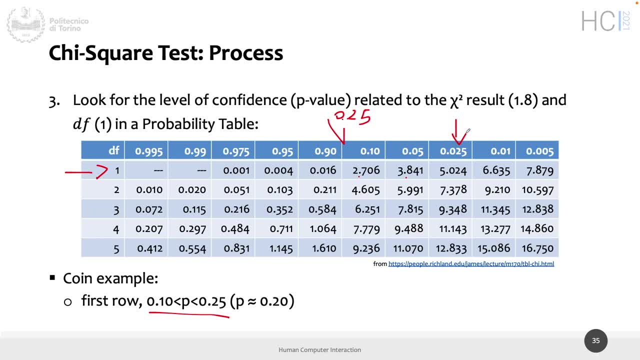 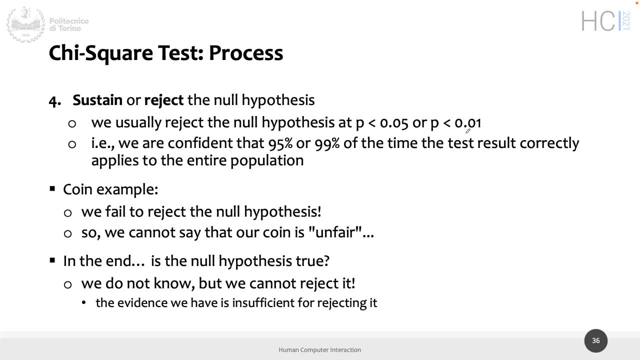 us where this number, given that the degree of freedom is in this table And we say, okay, it's around 0.2, more or less. So with this number, we can decide whether to sustain or reject the null hypothesis, And we usually reject the null hypothesis. 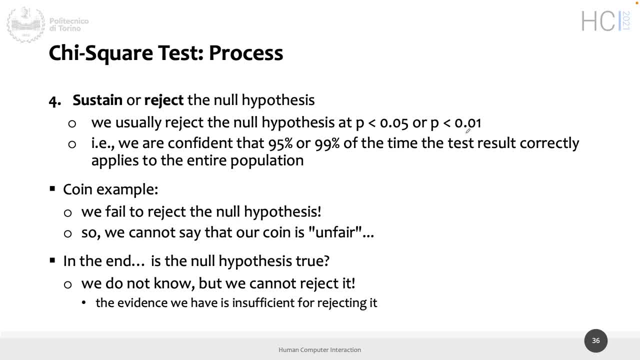 if that p value is minor than 0.05 or 0.01.. That means that we are confident, given the results, that either 95% or, if we look at 0.01, 99% of the time the test results correctly. 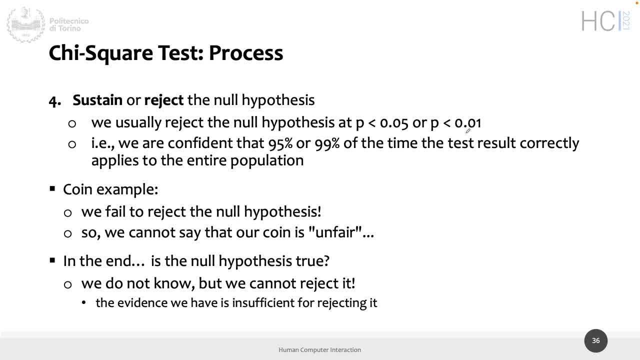 apply to the general population. In a way, we're saying, if we really do the experiment, we will see similar results. 95% or 99% of the time Depends if we use a p value of 0.05 or 0.01.. Clearly, 0.01 is more. 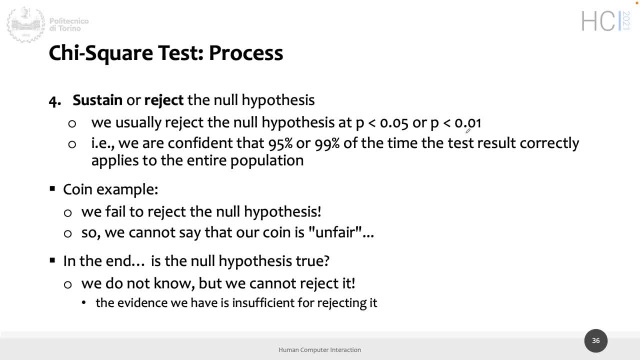 it's better because it's 99% of the time, so we are mostly certain that these results will stand. So in our example we have 0.01.. 0.02.. That is bigger than 0.05 and 0.01.. So we cannot reject the null hypothesis. 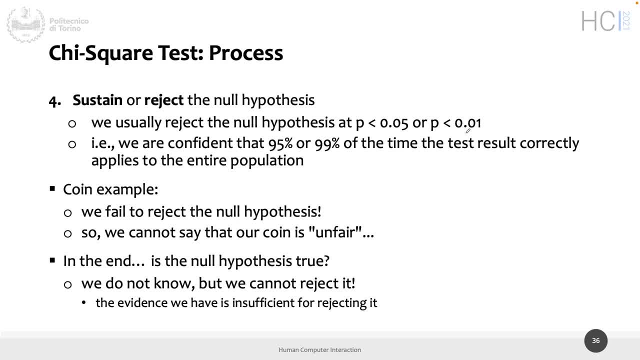 So we cannot say that my coin is fake, is unfair And thes. if we cannot reject a null hypothesis, we can demand awortыс, just say nothing. We can say: I cannot reject the null hypothesis, I sustain the null hypothesis. 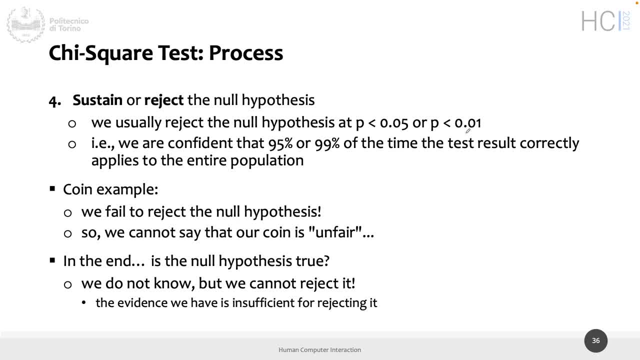 So we cannot say: notice that I'm not saying that my coin is fair, But I say that I cannot say that the coin is unfair Because this is the information that the analysis tell us. The analysis tell us that, with the data that we have, we cannot say that there is.